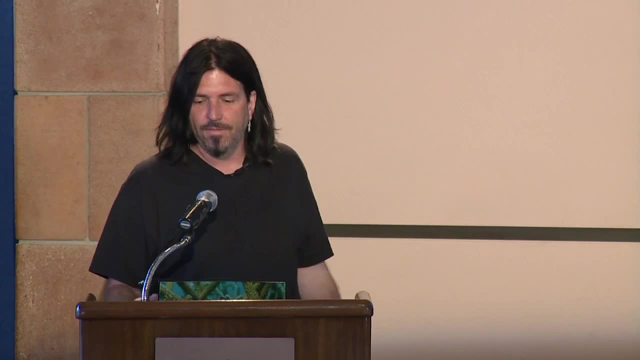 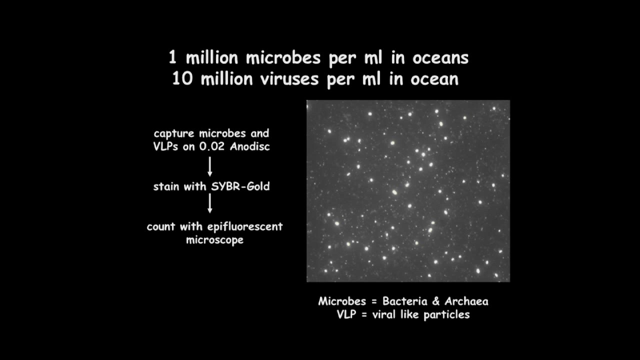 And that's because most of the organisms are actually the microbes and the viruses. There's about a million bacteria per mil in the world's oceans and about 10 million viruses. Those are the bacteria, and then all the little things are the viruses. For the most part, the viruses are actually. they are viruses called phage that infect the bacteria. 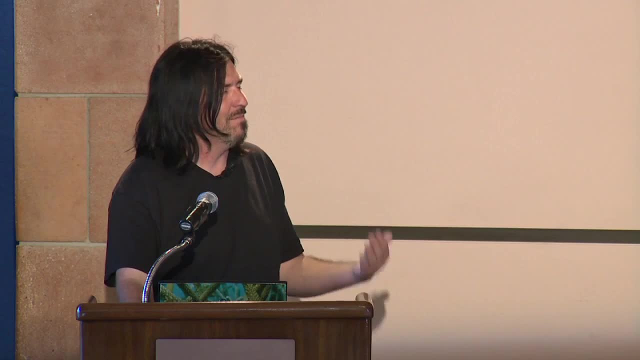 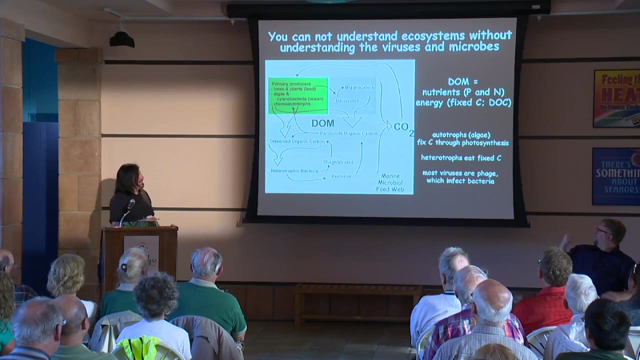 And they're one of the main controls on the types and number of bacteria that we have. Now, I hate to do this to you, but I'll just start with this. This is the really horrible thing, So you have to memorize all this. 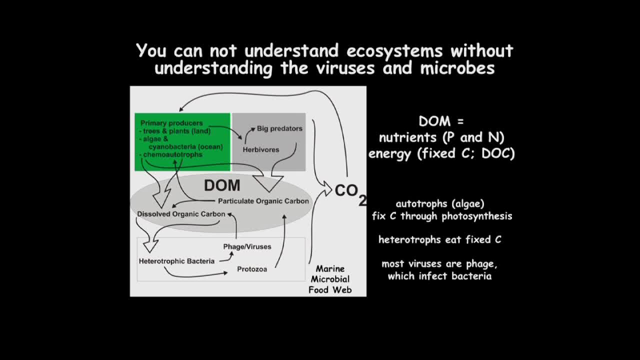 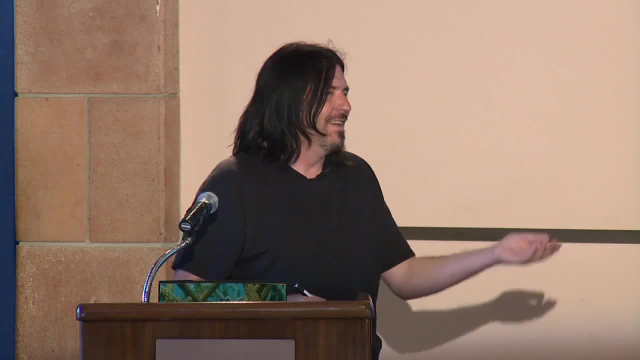 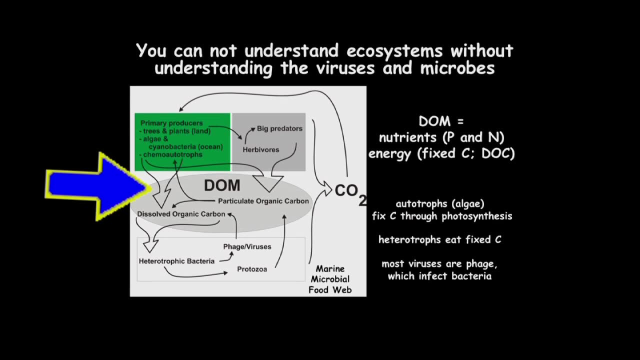 So the general rule of how the world works is that you have a primary production right. So these are your plants and your trees on land, grasses and, of course, algae out in the ocean. And what it does is it? It fixes carbon, and the carbon gets mostly shunted as sugar into this dissolved organic matter pool. To give you a feel, about half of the primary production that's done every day ends up either in the soil or in the water, And that dissolved organic matter feeds heterotrophic bacteria. And the heterotrophic bacteria are actually controlled. The number of them, the total numbers that you have, are usually controlled by two predator guilds. 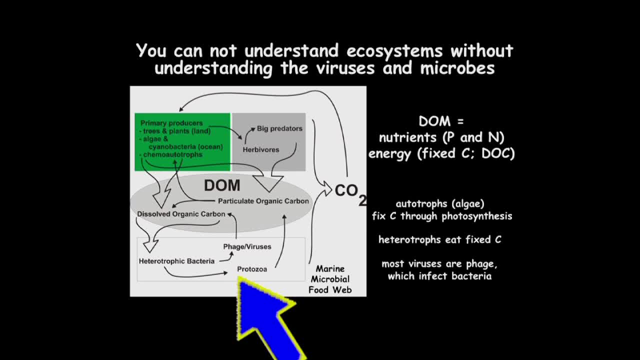 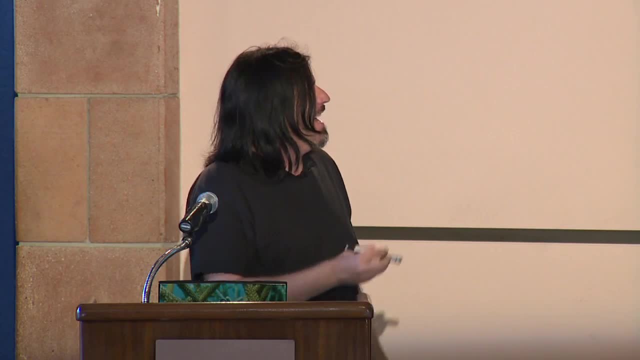 These viral phage predators And these nanoflagellate protists. The way everything is working out there is that, for the most part, the faster this part of the system goes, the happier. the microbes are Now. coral reefs, of course, exist in seas. And what they've got is they've got rushing over them this million bacteria per mil running onto the reef And they have to deal with all these microbes. Corals, of course, are really interesting. They are, For For all intents and purposes they're hunters, so they're cnidarians, so they have these nematocysts, so they reach out and eat zooplankton stuff by killing them. 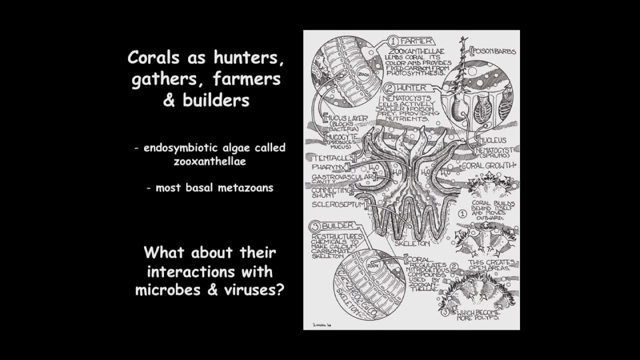 They're gatherers because they build the reefs right, So the reefs actually cause upwelling in different parts of the ocean and that brings up the nutrient-rich water from the bottom. They're farmers because they have these zooxanthellae, which are these dinoflagellates that live inside their tissue. 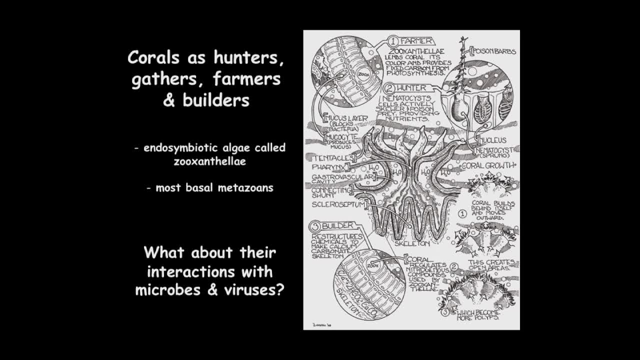 And it allows them to Harvest energy via photosynthesis directly. And then finally, of course, they're the builders of the reefs, And they build these structures, which are the biggest things, actually, that ever build on the Earth- by a fair amount. 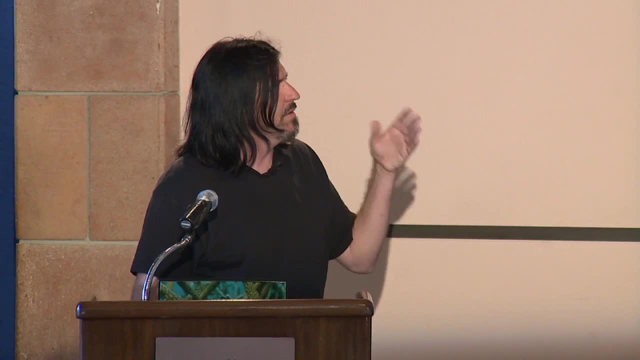 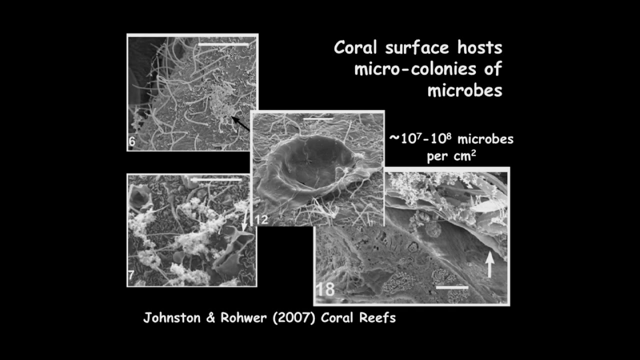 And one of the main questions that I started with was just what's the interactions between corals and this microbial part of the world? This is what an electron micrograph would look like over the top of a coral. This is also basically how your lung would look, just so you know. 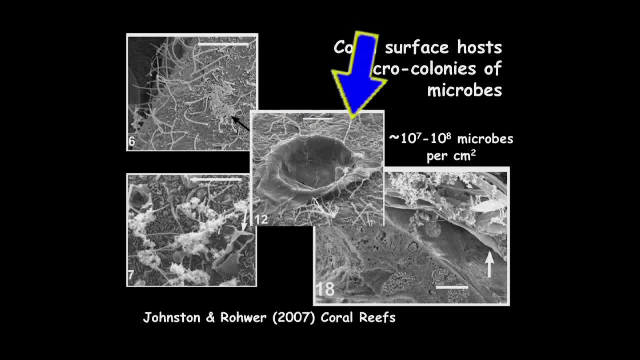 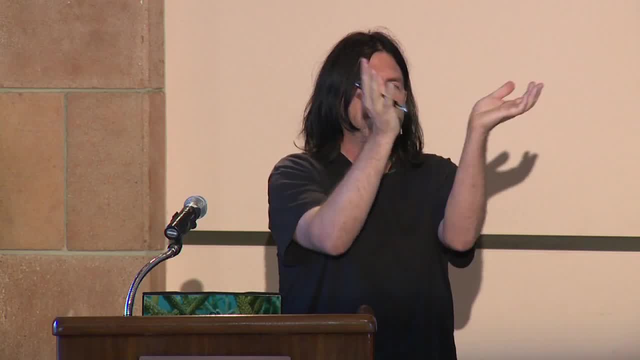 Mm-hmm, So Mm-hmm, What you have is the tissue here, and then you'll have: These are the cilia, okay, And then this is a mucus bubble, And what's happened is that the mucus bubble comes up like this and then it's actually collapsed because of the way we've treated the sample. 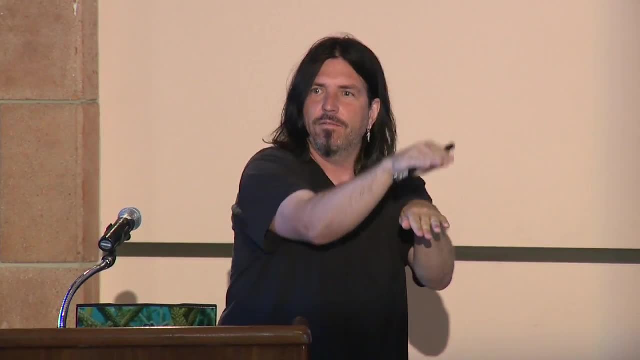 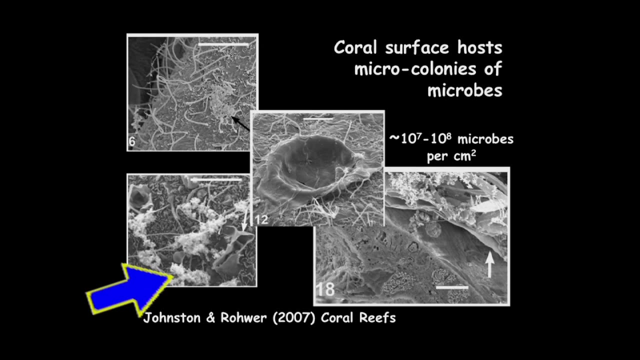 So normally that would pop up and then the cilia would knock it off. okay, That's how you clear your lungs. It's how a coral surface clears itself of bacteria. The bacteria look like they actually live as little tufts or little microcolons. 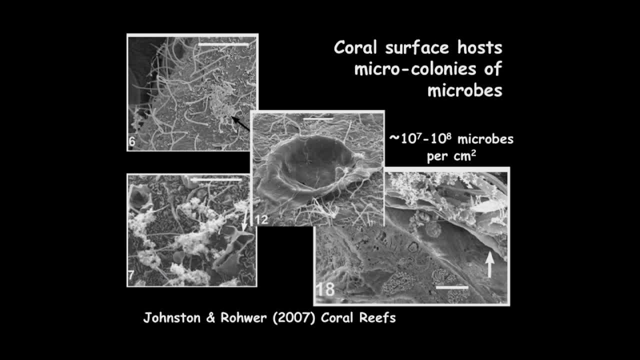 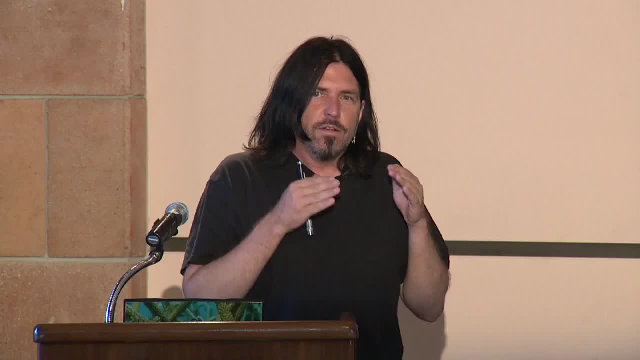 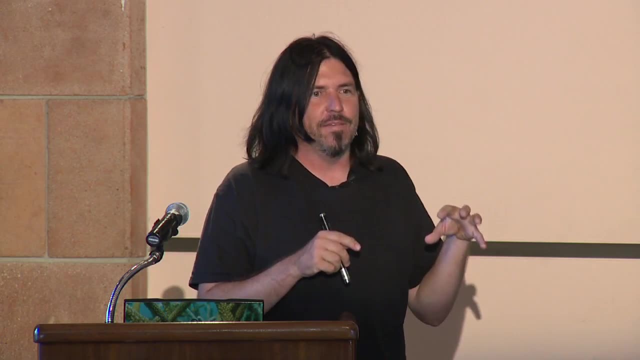 They live as little colonies on the surface, but they're actually never touching the coral. So you can see, here there's always a protective mucus layer between them and the bacteria on top. Coral microbial interactions, or specifically the coral bacteria interactions, are specific. 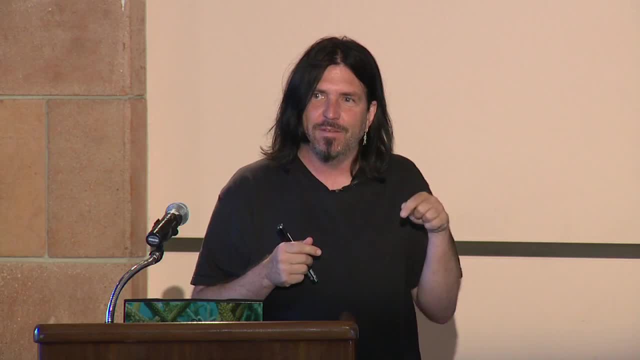 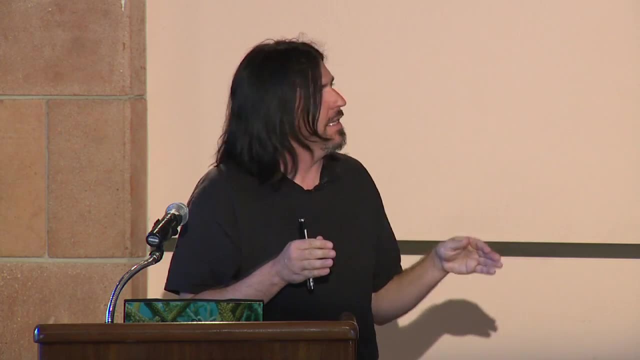 It's the same with people. So you guys have specific microbes that are different from apes, for example. okay, Corals are the same way, so, even though they're sitting in thisin water, where you'd think, oh, they can- justa microbe can move from one to the other- it's actually not true. 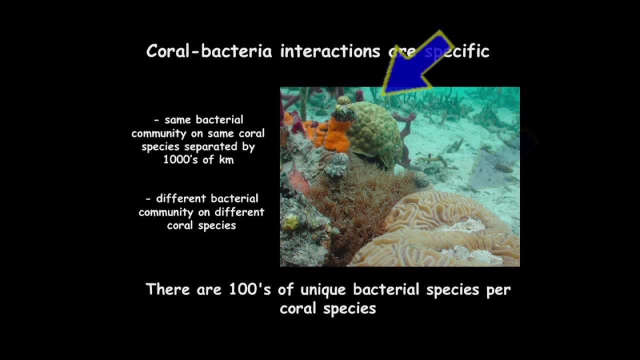 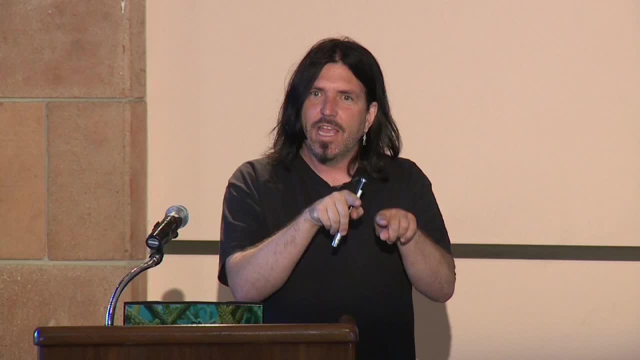 So this coral right here will have completely different microbes than this one right here, And it doesn't matter: even when they're touching each other, they'll have totally different microbes. Each coral will have hundreds of unique bacterial species on it, right? 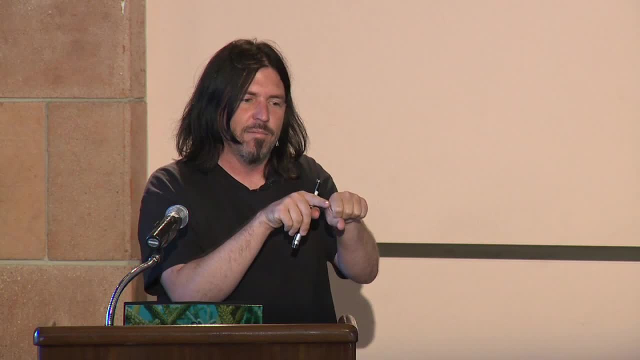 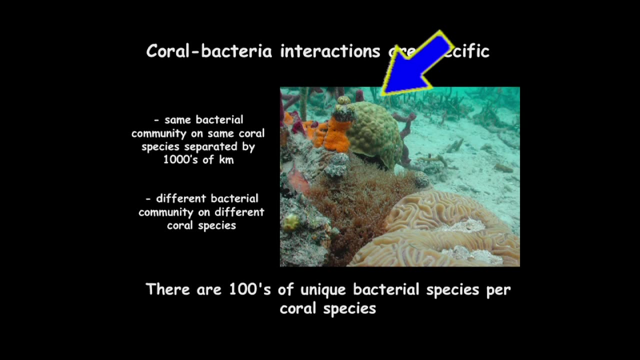 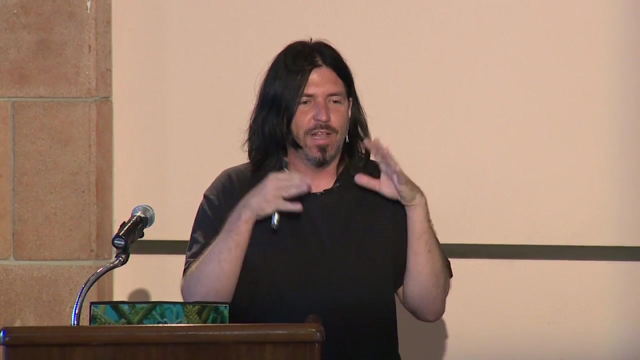 So most of the diversity on the reef is actually the microbes living on these different surfaces. Now, if you look at this coral 1,000 kilometers away, What you're gonna find is that it has the same bacteria. So you can look all over the world and you can find that one coral species will have. 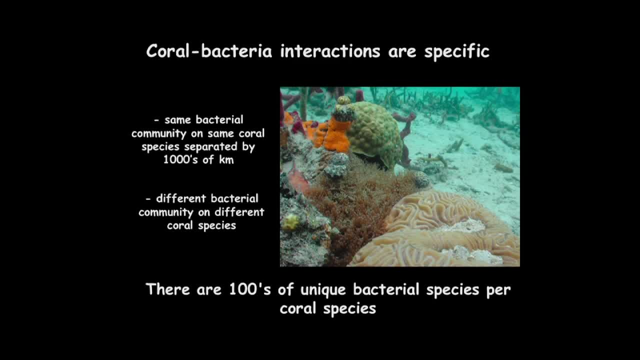 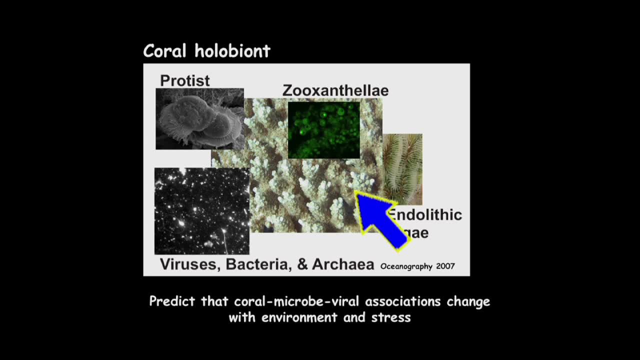 100 different types of unique bacteria, and they're only specific to those corals. If you take all this together, you build something that we call the coral holobiont, And what that is is it's the coral animal with the zooxanthellae, the algae that live. 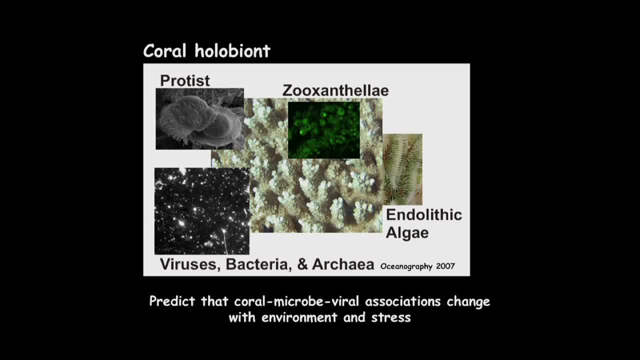 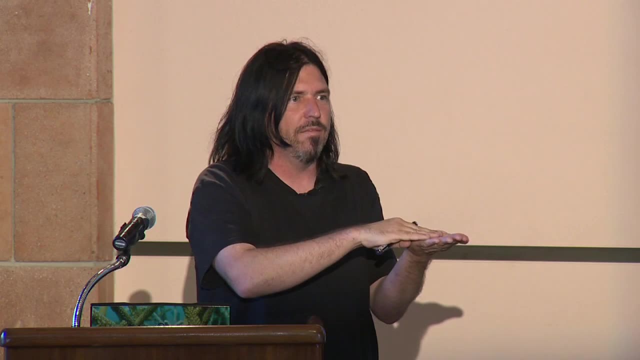 in it. okay, And these can change depending onthe same coral can have different types of these: The bacteria and the viruses. most of the diversity is gonna be here, as well as the protists that live on top of them, And in this coral skeleton you'll actually have this indolithic algae and indolithic. 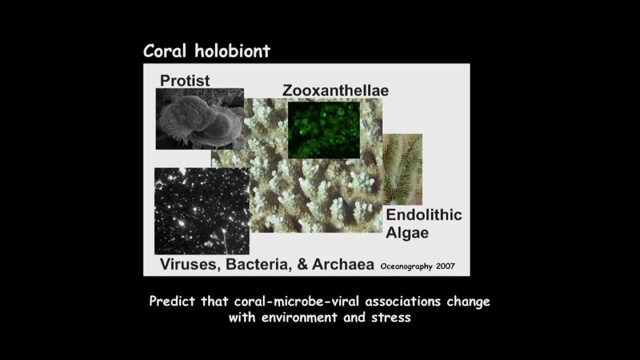 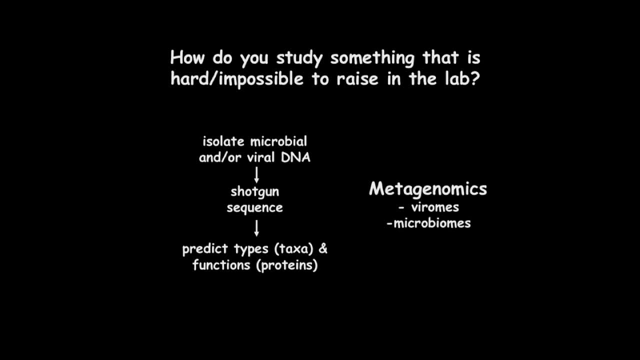 fungi that lives in there, And these guys exchange nutrients, they exchange genetic information. there's a whole bunch of stuff going on in there. Now the question becomes: how do you actually study the microbes and the viruses on corals? And why that's always been difficult is because, for the most part, you can't. 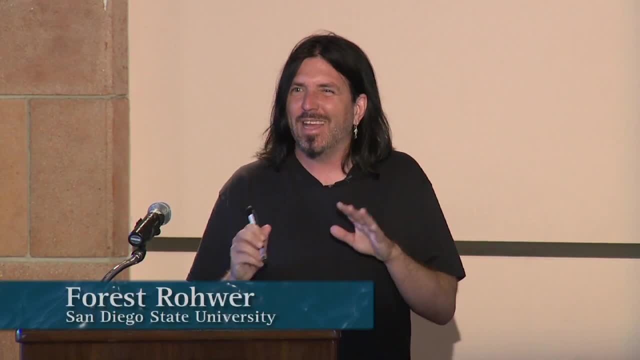 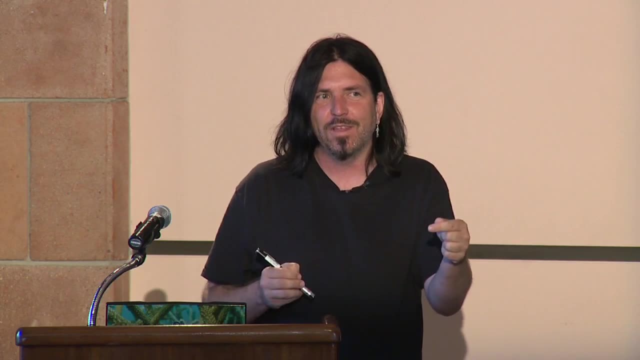 You can't culture most of the microbes out there, okay, And that's about 98, 99% of them. And it's even harder to study the viruses, because to study a virus you have to culture the thing that the virus is gonna eat. 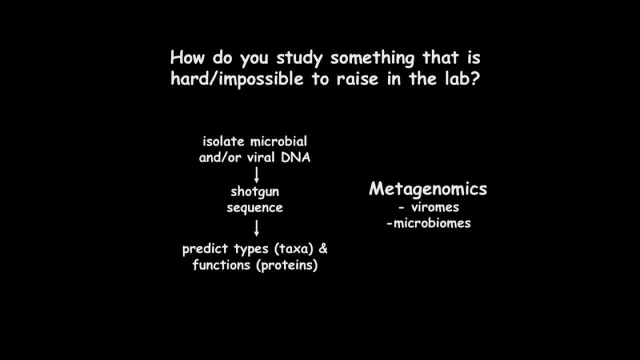 So you can imagine most of the viruses we've never studied, And the way we actually do that is we just go out to a system- and this was invented at Scripps for the most part- and what we'll do is we'll isolate microbial and viral DNA. 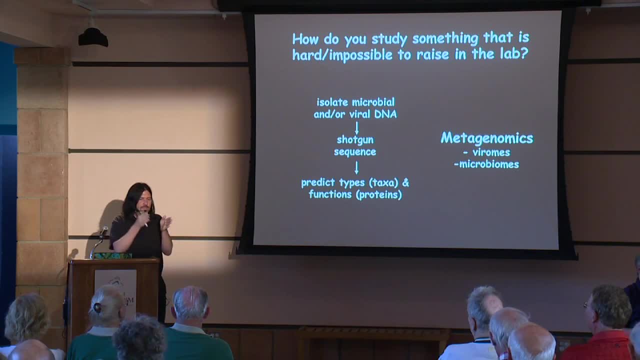 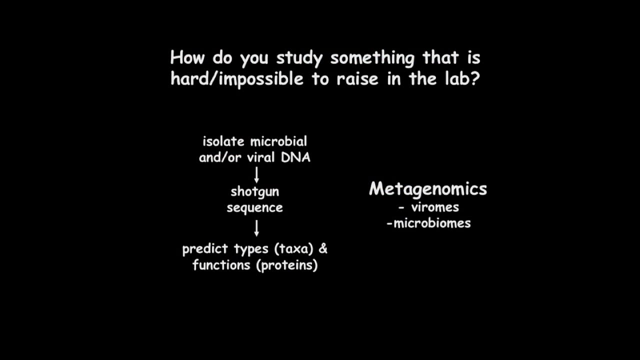 take the DNA, We're just gonna sequence it, So we're just gonna get the code for all the different pieces of DNA there And then from that we can predict the types of microbes that you have and what sort of genes they're encoding, right? 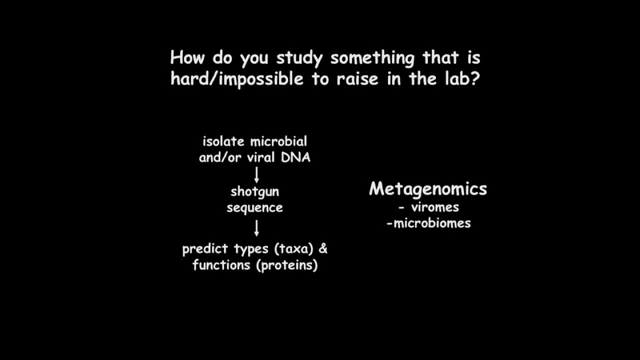 Does that make sense? And this is what we call metagenomics, And you may hear me say viriomes or microbiomes, just so you know, Sometimes I fall into the jargon. That just means the viruses or the microbes. And this is how you do it with a coral. 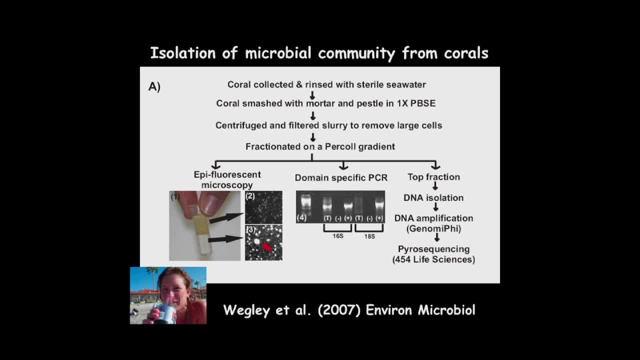 You take the coral, you blend it up, And then you take the slurry And you fractionate it And what you get is the microbes on the top, And then the zooxanthellae in the coral tissue is actually at the bottom. 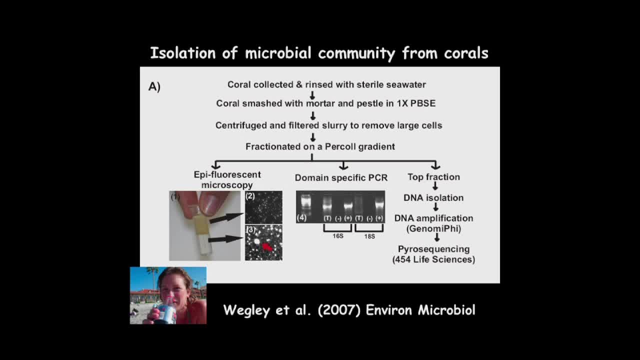 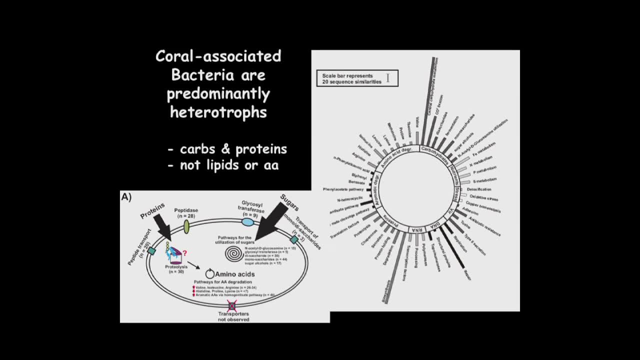 If we take this, then we'll go and sequence it and we're gonna ask: what types of microbes do we have there? And from this you can actually figure out. what are they doing, How do they interact with each other. And what is important in this figure right here is that most of the microbes that we 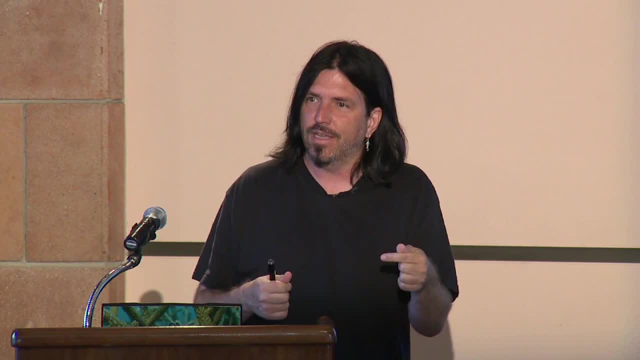 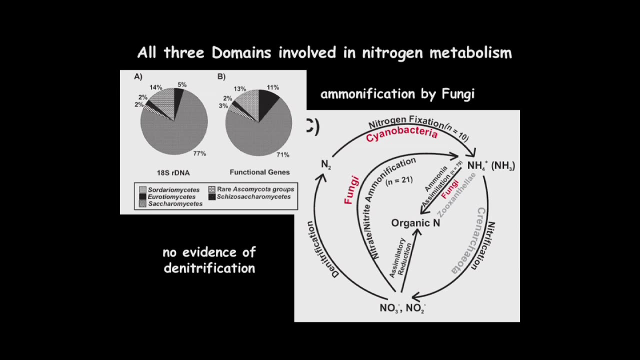 find on coral are actually just eating the mucus that's associated with it. That's what their main job is. So what is going on on the coral and what you learn accidentally with some of these approaches is that the coral and the microbes living on them actually form this really amazing. 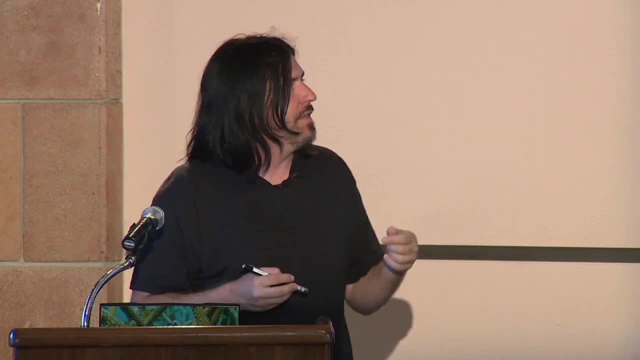 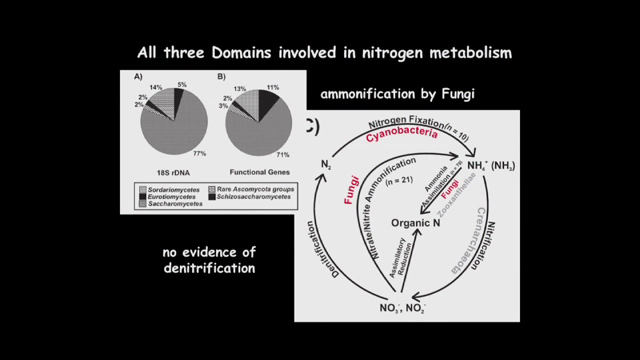 system where they can manipulate the nutrients that are coming in. So most coral reefs occur in nutrient-limited environments, And so one of the main nutrients that they're missing is nitrogen. Okay, I don't have to remember all this, but I just want you to follow this a little bit. 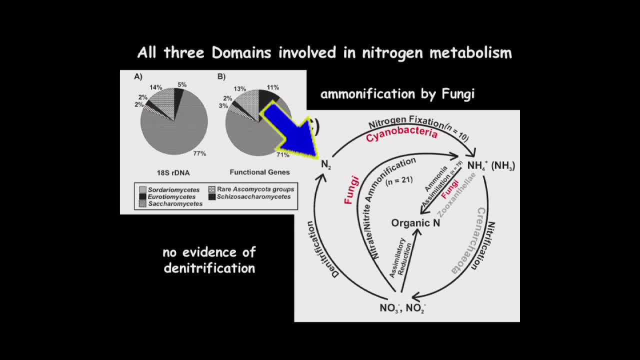 So if you take gaseous nitrogen from the atmosphere, there are living on corals cyanobacteria which can fix the nitrogen. They can make ammonia, which then can be denitrified by a whole different group of microbes called archaea. 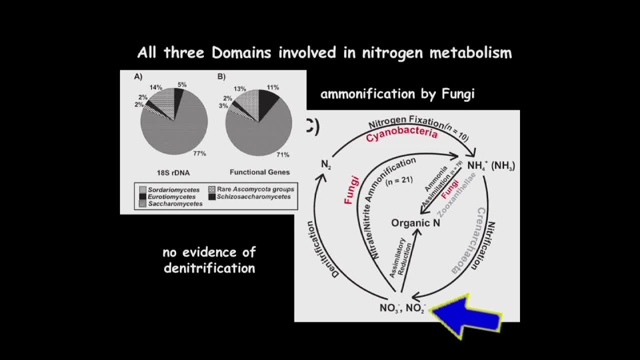 And then, instead of losing the nitrate and nitrite, which would normally be put off as gas, But actually there is fungi that change that back to ammonia, So they recycle the thing. So this is all three domains of life actually working together to recycle nutrients within. 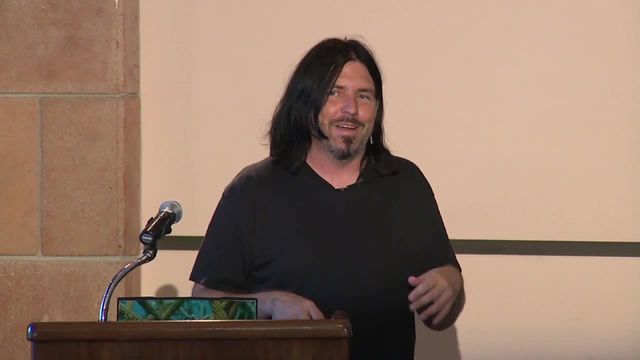 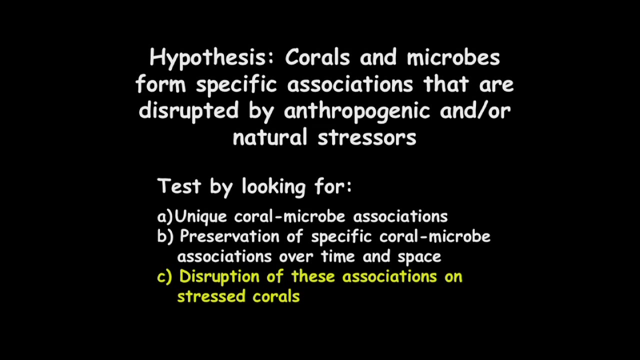 the coral holobiont. That's the good stuff. Now I'm going to get into the depressing part of it. So here is our hypothesis. Remember, we've shown basically, corals and microbes form these specific associations And one of the predictions is that these things can fall apart when you stress the system. 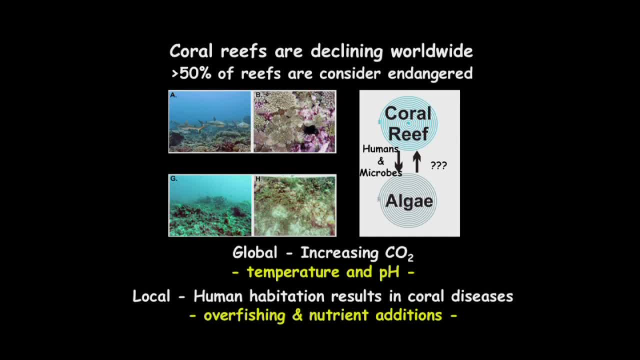 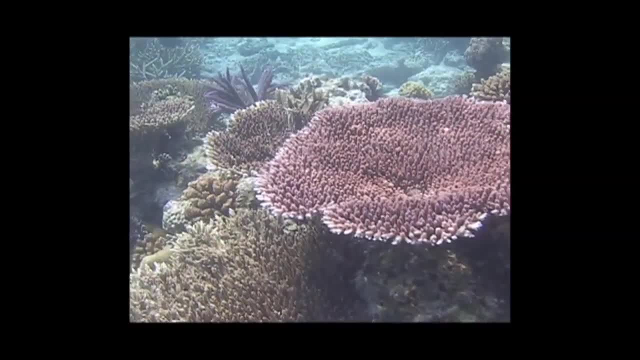 Of course, you know that coral reefs have this global decline, And I'm just going to show you what that looks like. All right, So this is a coral reef. This is actually in the Indo-Pacific, And what I really want you to notice here is that you have a whole bunch of different. 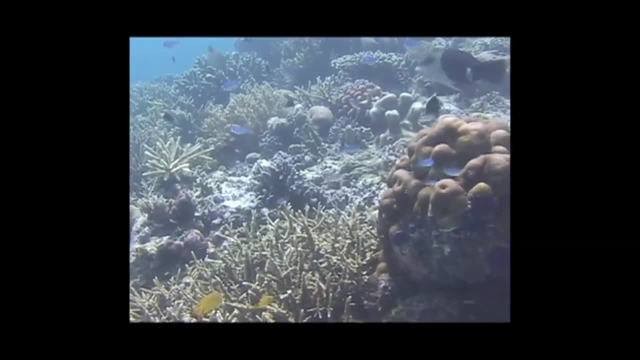 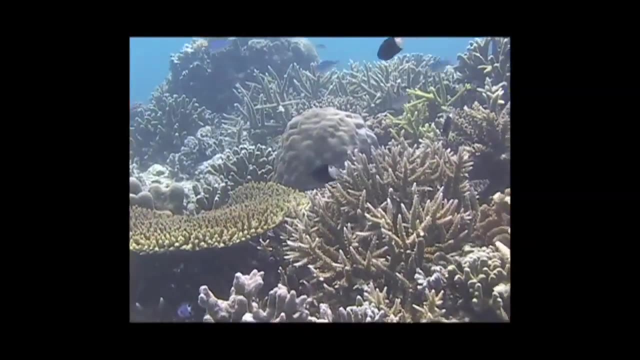 coral types. They form these massive three-dimensional structures, So you can see they're basically competing for space with each other. There's a lot of different fish and a lot of different types of fish. There will actually be a lot of big fish eating all the small fish which we'll come back. 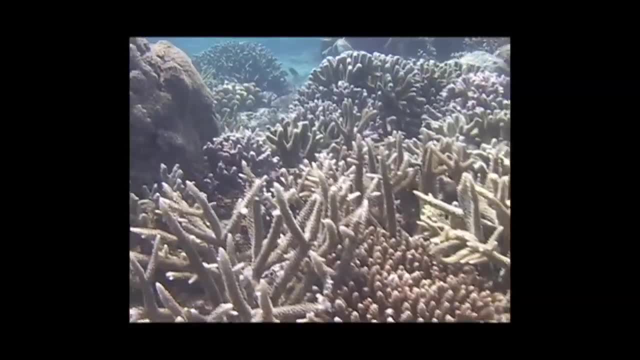 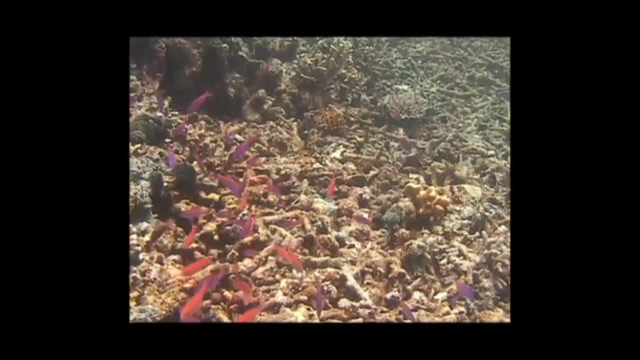 to in a little bit. So this is the site. And then we went back to it five years later And this is what's happened to it And you can see, you lose all the structure. So all the coral has died by now. 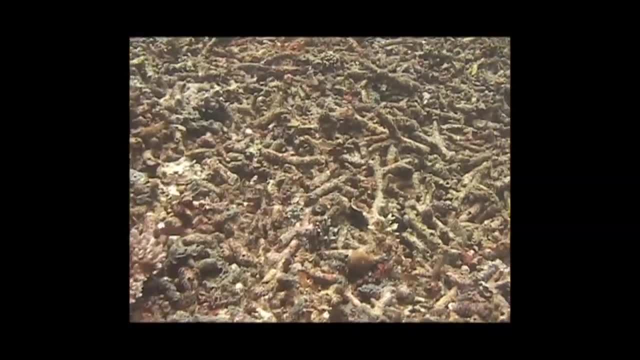 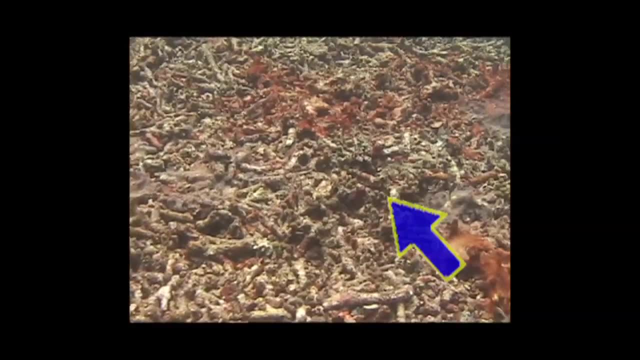 And this is all covered with a type of algae that we call a turf algae. So this is just a microscopic algae for the most part. You've lost most of the fish, especially the big ones Right there. that's just a microbial mat, just to let you know. 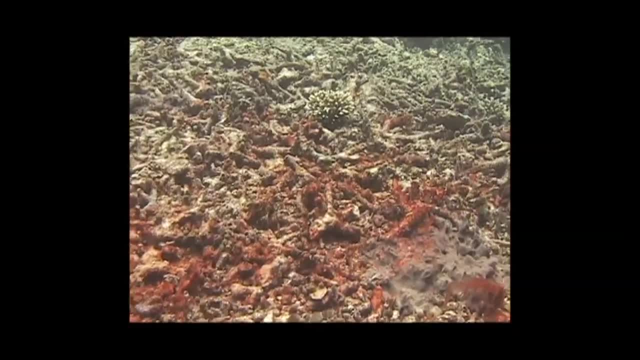 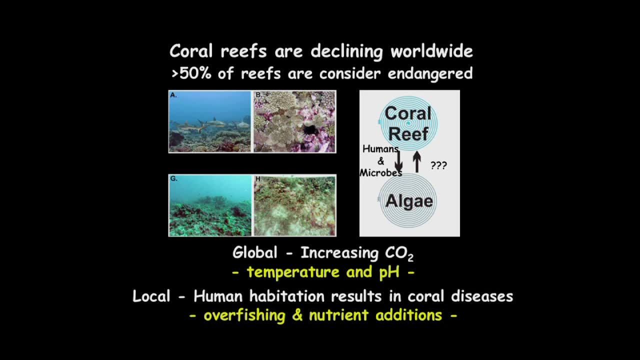 And that's what's going on essentially all over the planet- And we think, of course, that it has something to do with people- And the main considerations have been the changes in CO2 on the environment, The idea being that maybe we're changing the temperature and the way the temperature is. 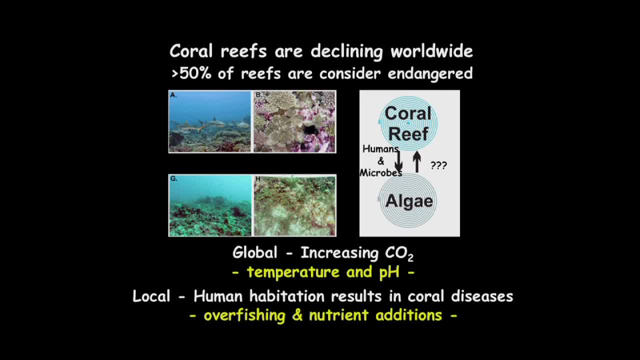 distributed across the planet And that leads to probably the most famous, which is: if you increase the temperature of a coral, it causes coral bleaching when it loses its nose and belly. The other one that we're getting That people are concerned about, of course, is acidification. 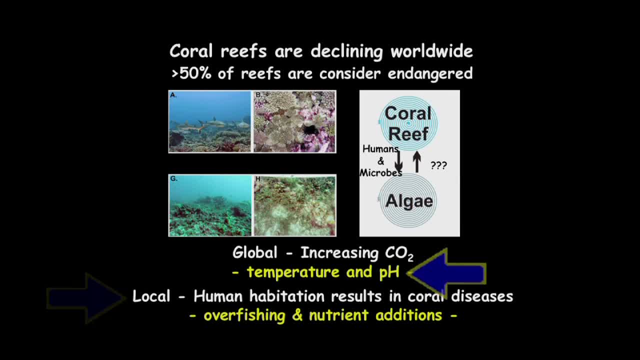 Because as you add CO2, you actually change the pH of the oceans. And then, finally, there's this thing, which is what I'm mostly interested in, is there's something about local. So if you put people on coral reefs, they start dying. 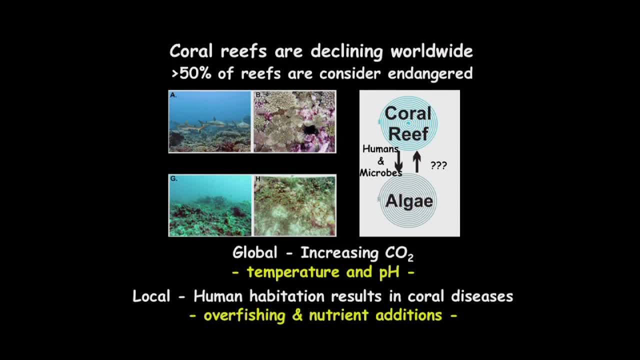 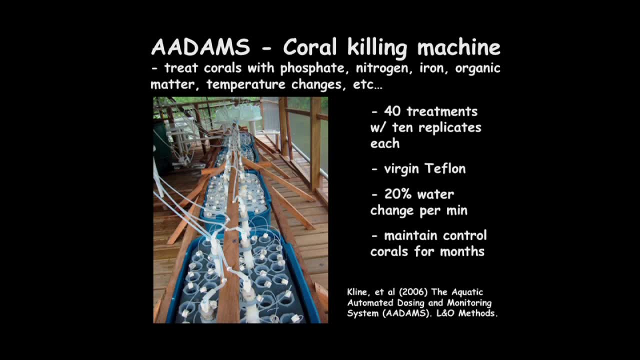 There's something about people that kill coral, And we think it has things to do with overfishing and nutrient additions, And this is the one I'm mostly gonna talk to you about today. This is an experiment that I ran when I was at Scripps with Nancy Knowlton. 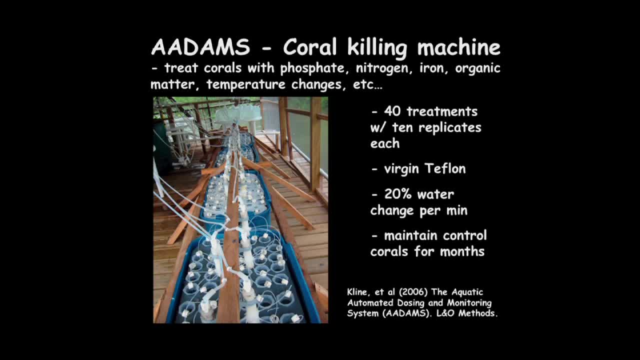 And we built this system down. Davey Klein and I built the system down in Panama And what we did is we put little- Each one of these cups has a little coral nubbin in it- And then we take water right off the reef. 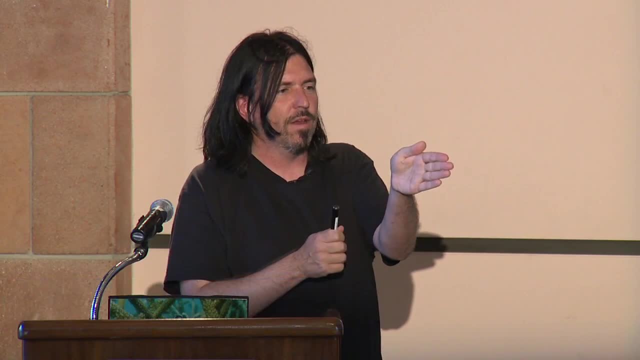 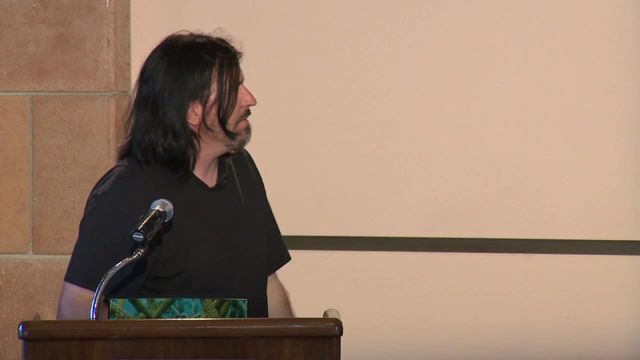 And just as it's running into the coral. where the coral is, we'd add some treatment of some sort. Okay, So we're gonna test all these potential things that might be killing corals. And the surprise was: What? What? 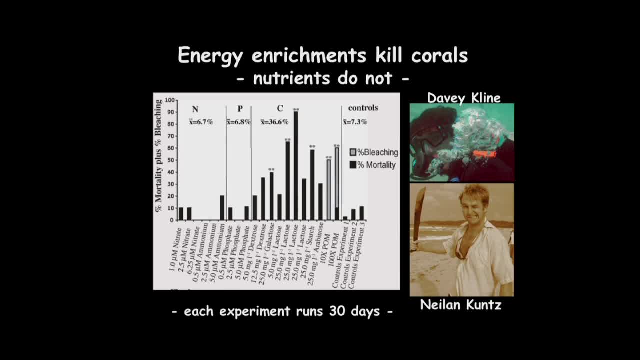 What? What's the problem? What's the problem? What's the problem with that? And I did a luminescence test with the corals and they showed some things that kill corals. But the only thing that actually killed corals directly in this experiment were additional. 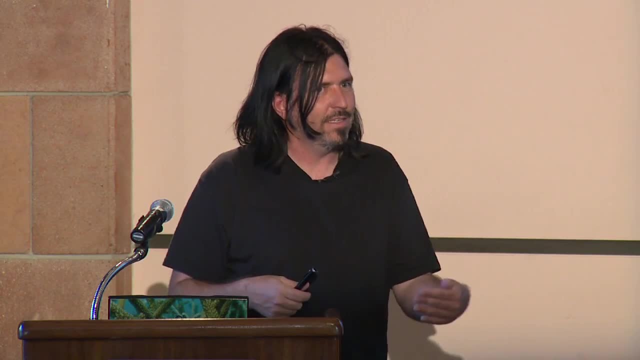 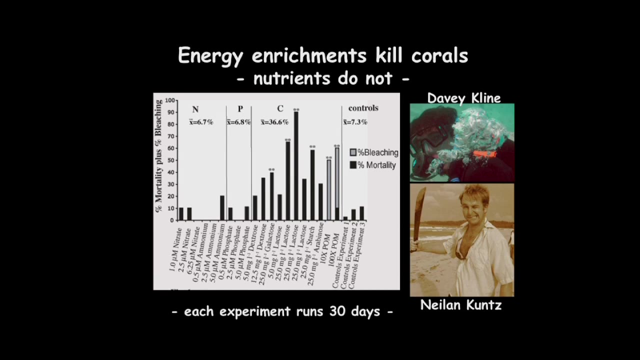 carbon sources. The nutrients didn't do it, pH didn't do it, a whole bunch of other things that we. So these are these different carbon sources And it really doesn't matter what carbon source you use. You could use naturally occurring carbon sources, things you buy from the chemical company. 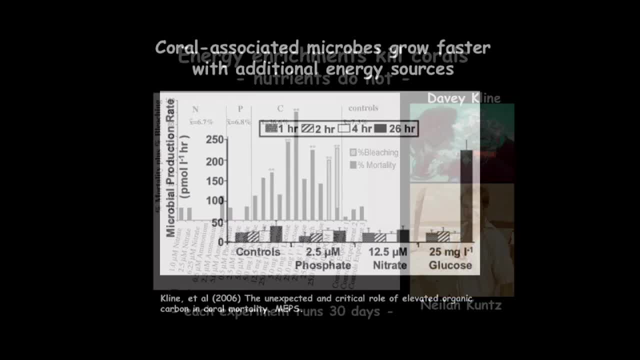 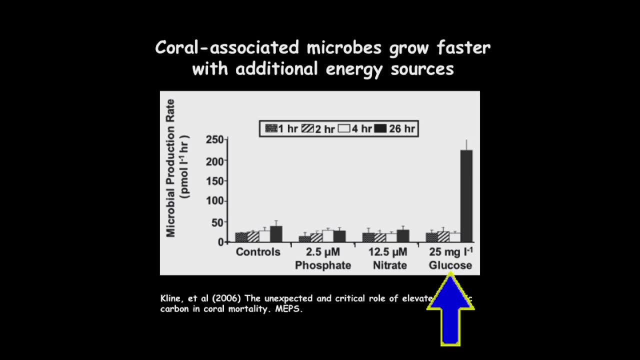 etc. And all of them would actually kill the corals. The other thing that happened is that when, But when- we did the- This is the carbon source treatment here- When we did this, this is the growth rate of the microbes associated with the corals. 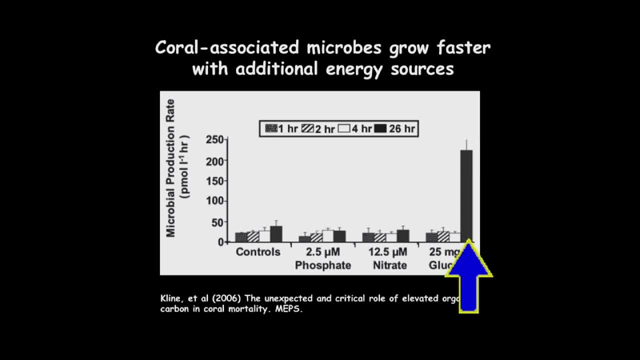 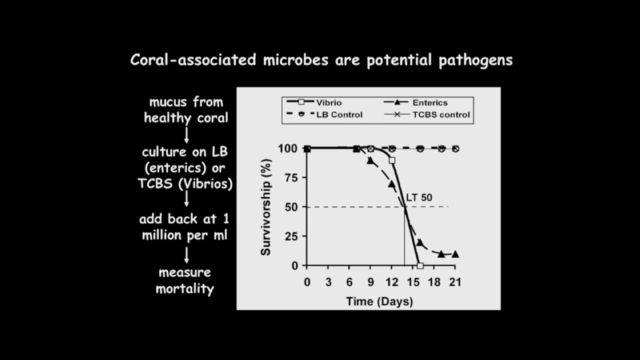 We saw this change in the amount of coral, the rate at which the corals are growing. So all this suggests that what we're doing is we're actually changing that relationship between the coral and the microbes that live on them. So if you take some of the specific bacteria that live on a coral and we 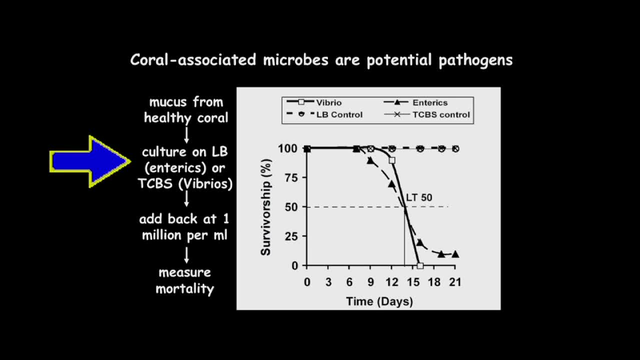 That's just a way of culturing them up. on LB or on TCBS You come up with these two different bacterial groups And if you add them back at a higher concentration than they're normally on the coral, they kill the corals. 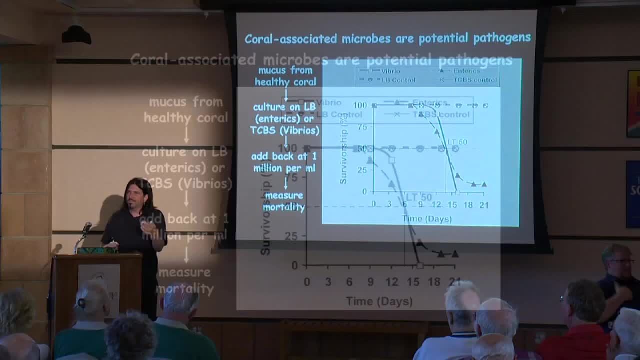 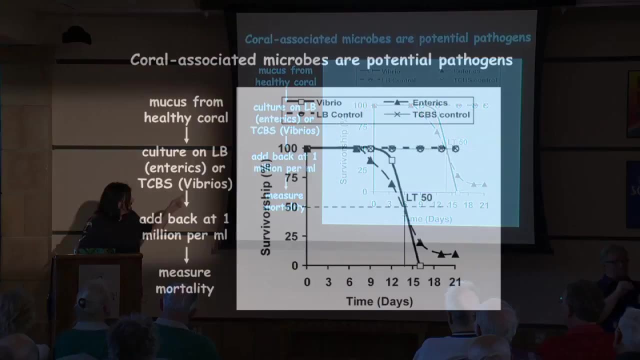 So the bacteria that live on the corals are actually able to kill them. That's true of you. You're probably About a third of you are carrying a microbe that will kill you in the end. That's what's going on here. 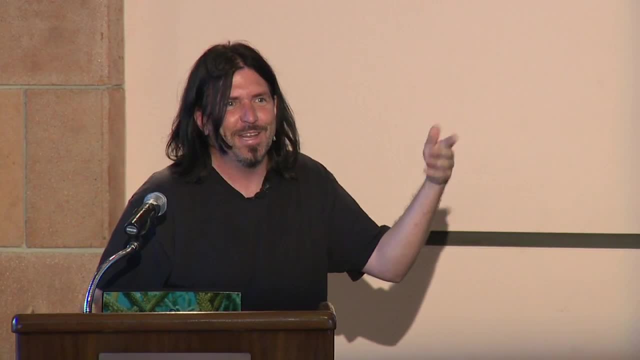 It's good to know At least you've been carrying them, feeding them, and now they'll get you. So that's a way of culturing them up on LB or on TCBS. You come up with these two different bacterial groups. 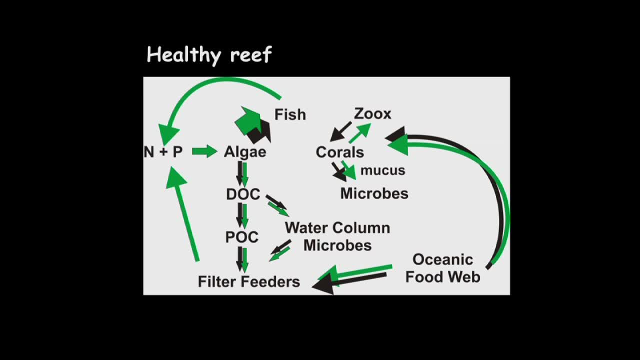 And if you add them back at a higher concentration that they're normally on the coral, they kill you like children. So what that means is that you've got the Normally on a coral surface. you've got these microbes that are living there. 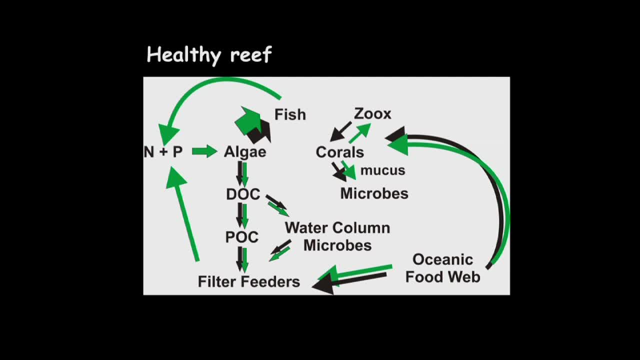 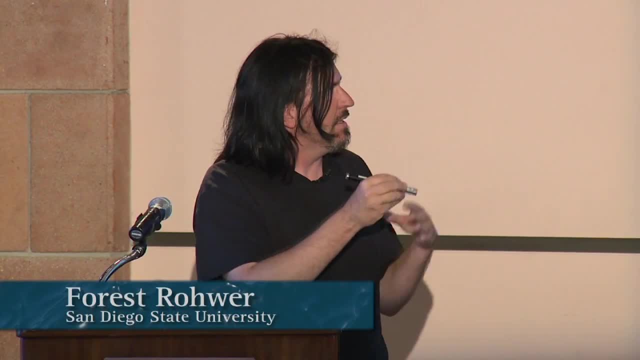 They can potentially come back and get you, but for the most part, you're controlling them, and we think you're controlling them by the mucus that you're feeding them. Now, if we go onto a reef, how does this all go together and how do we understand how microbes 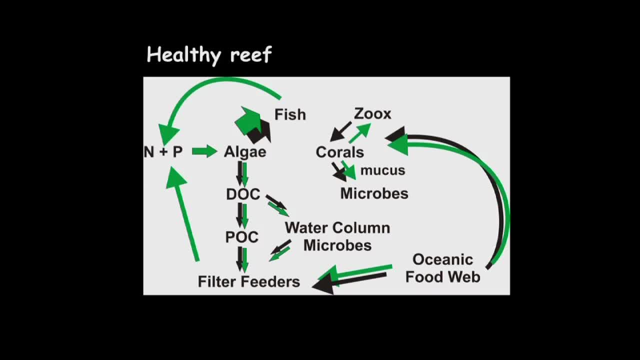 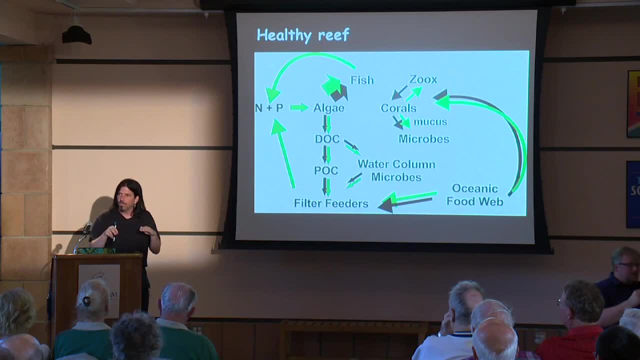 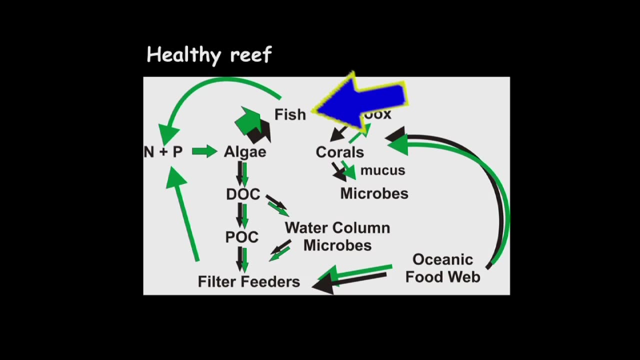 might be influencing reef dynamics On this healthy reef. Once you go to the algae, you couldn't actually see it. So if you go to a healthy reef, all you essentially see are coral and surfaces where the fish have been grazing. That's because the algae is grazed extremely fast by the fish. 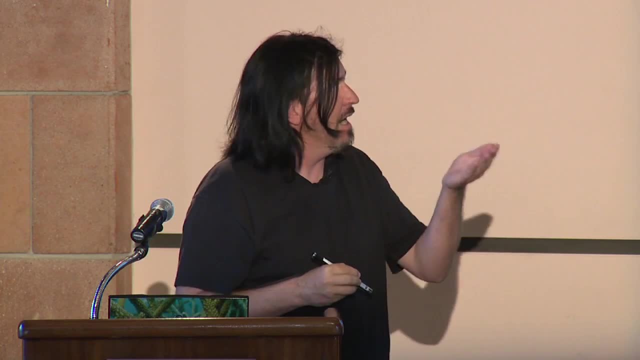 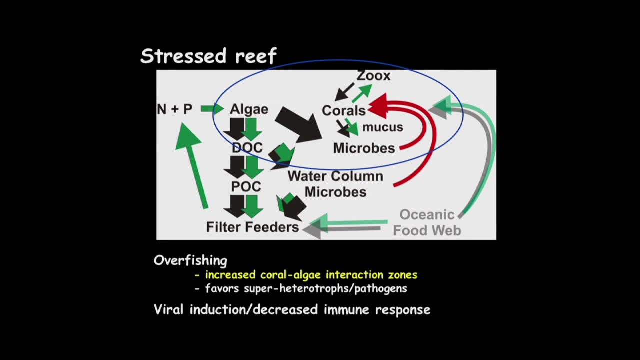 And so you're always moving the sugars from the algae up into the fish And the first thing that we do is we come along and we eat the fish And what that does is that allows the sugars from the algae that add to the dissolved organic. 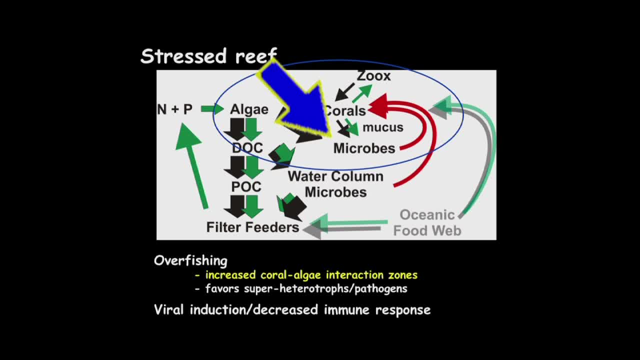 carbon, which can either feed the microbes that are already living on the corals- the ones that we've seen can kill them- or they're actually feeding the ones in the water column, which could potentially come back and attack the corals also. 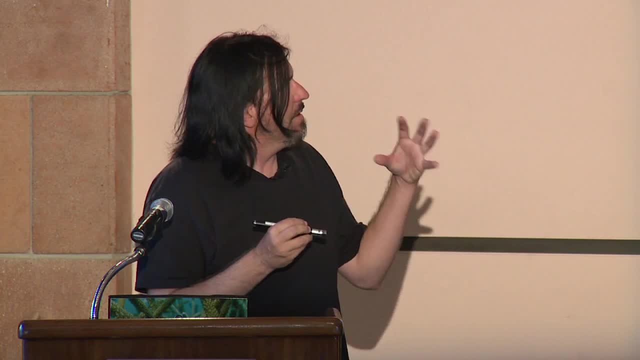 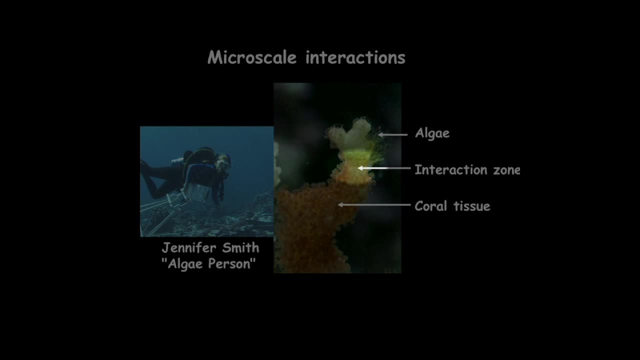 So does that happen? I'm gonna show you a couple experiments where we actually looked at right where algae is growing next to coral. So what we're gonna be interested in is this zone right here. So this is an algae that has not been grazed down, so it's growing up to be bigger. 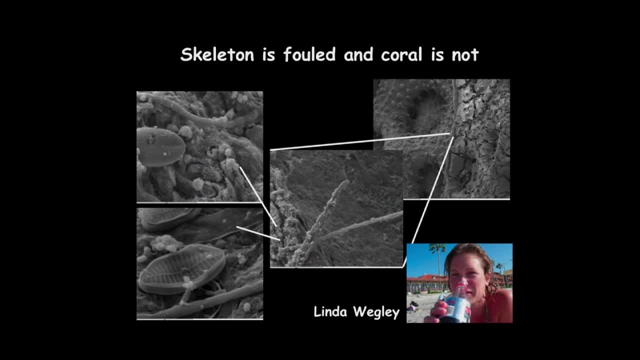 Okay, And it's starting to kill the coral. And if you look right at that interface, what you'll see is that the coral surface right here is still basically microbial-free, like we saw before. But right up against where the algae is, you can see these massive microbial maps right. 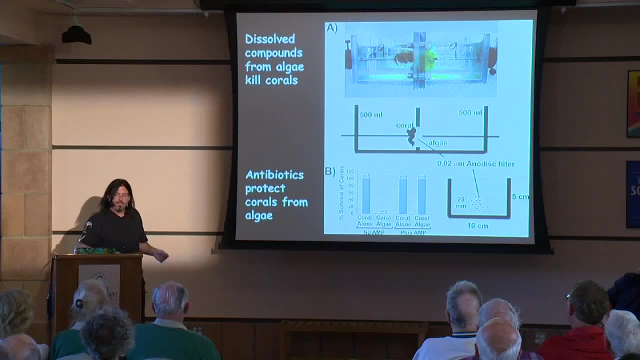 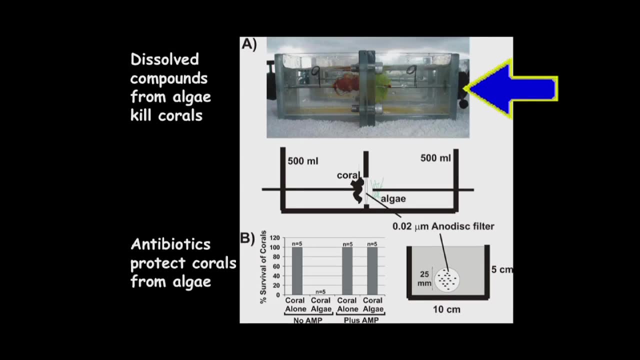 So all the microbes are right up against the coral And if you just stimulate that in the environment. So now imagine, what we're gonna do is we're gonna put coral next to algae in these little things here And we're just gonna watch what happens to the coral when it's across from the algae. 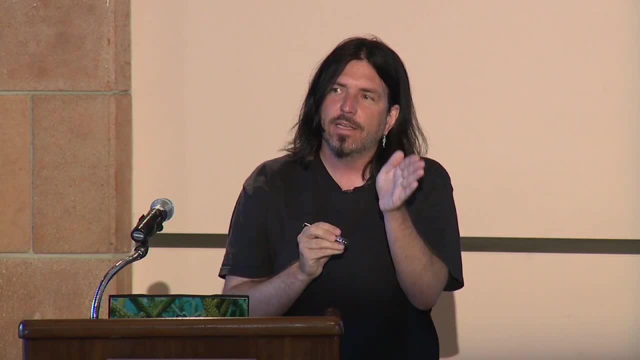 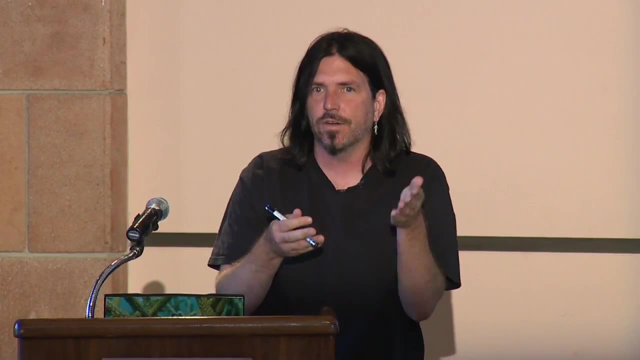 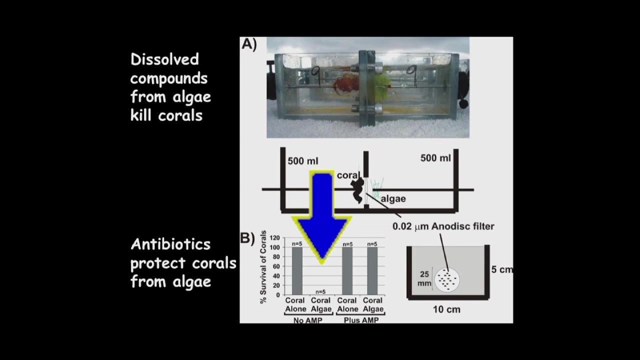 And between them we're gonna put a filter, and the filter blocks viruses or bacteria from moving between them, So the only thing that can move are things that are dissolved in the water, like sugar or something of that nature. When we do this, coral across from algae, all of the corals die. 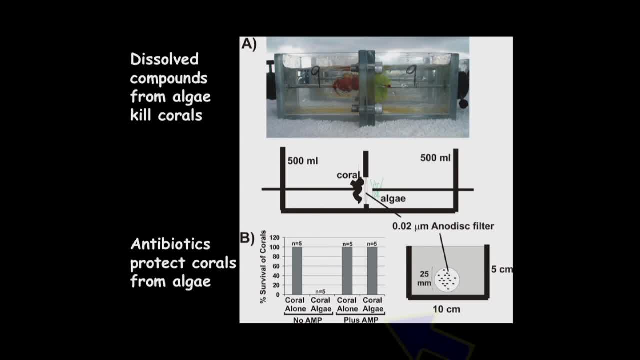 Coral by itself. it's fine If you do the same experiment and you put coral across from algae: all of the corals die. Coral by itself. it's fine If you do the same experiment and you put coral across from algae: all of the corals. 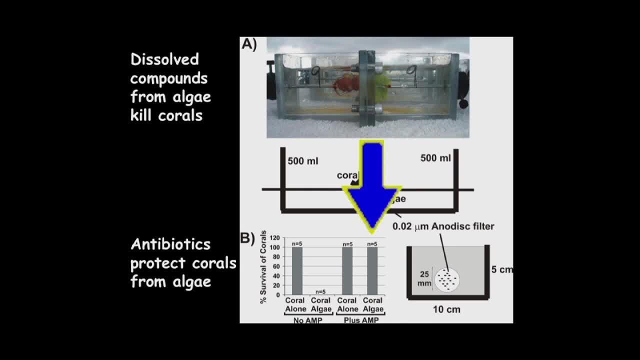 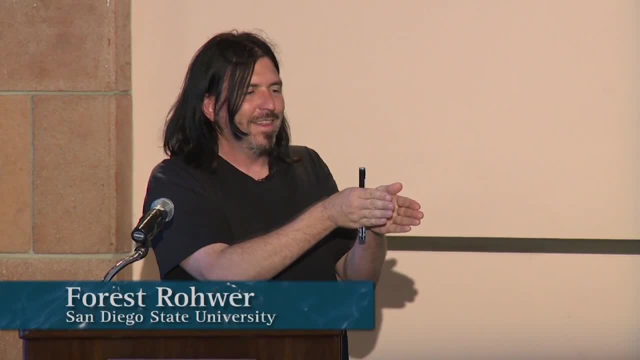 die. But now you add an ampicillin, which is an antibiotic. all of the corals live right. So what that tells you is that there's something coming from the algae that's associated with microbial activity that can kill corals directly. 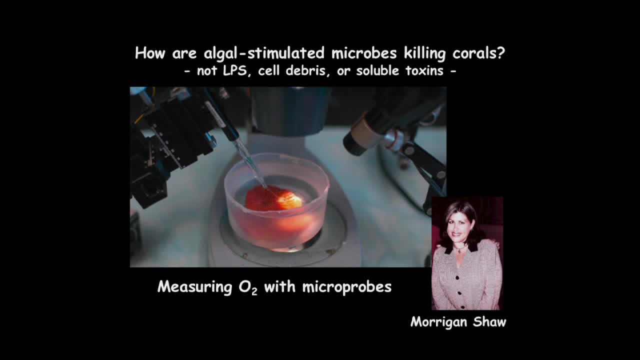 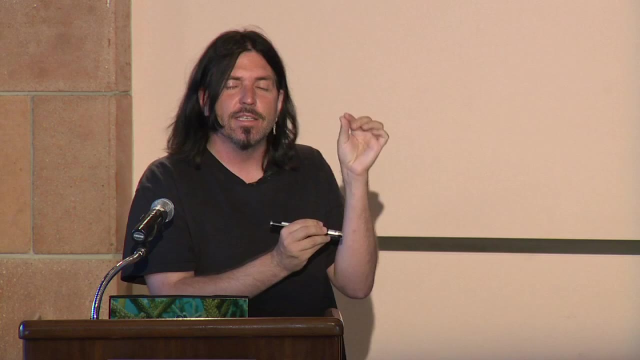 The way we think it's working, after lots and lots of different false starts, is basically they're just suffocating the coral, it looks like. So what's going on here is that this is a microprobe And you can go in and you can actually look at oxygen gradient at about a millimeter to. 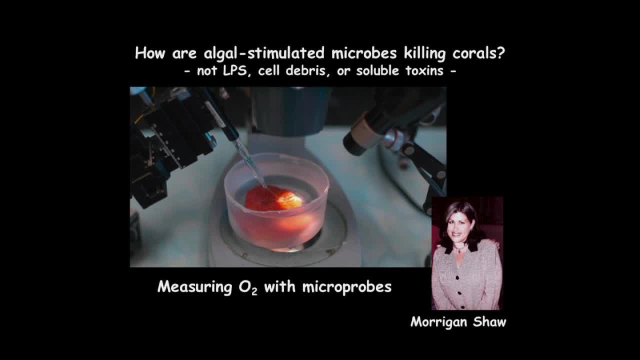 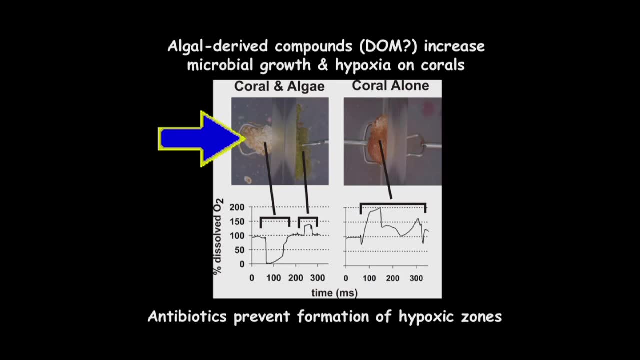 a micron scale, And so we're gonna go in and we're gonna look at where the coral's dying and we're gonna measure the amount of oxygen there. If you do that, if you go back to that experiment where the coral was dying here across from, 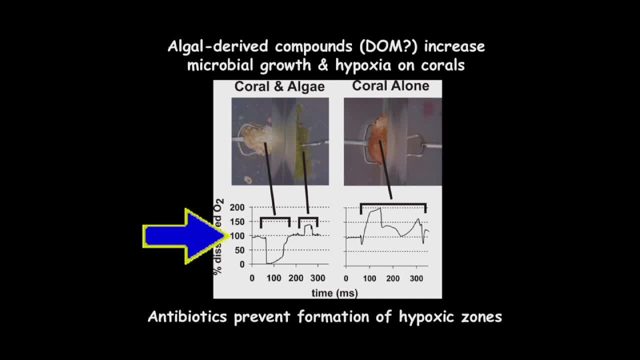 the algae. what you can see in seawater, that's our 100% dissolved oxygen. Okay, So here you go to the coral, across from the algae. it goes totally hypoxic, so there's no oxygen there, And then when you get back to seawater, it's 100%. 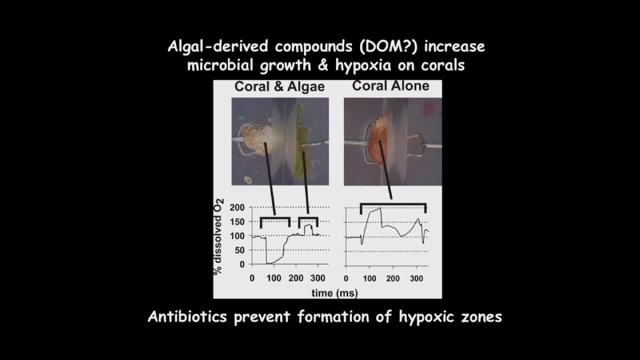 And then when you get across from the algae, it goes higher. That's because the algae is actually doing photosynthesis, so it's producing oxygen. The same is true of coral by itself: it produces oxygen when there's nothing across from it. 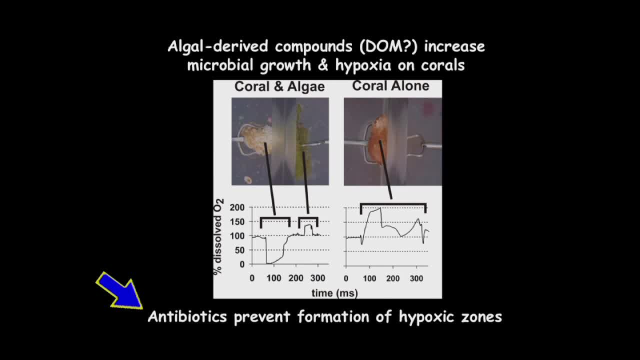 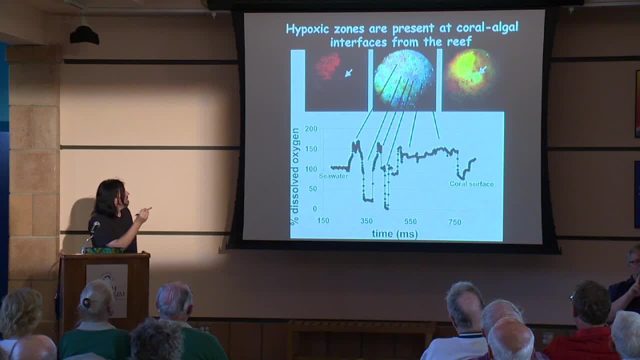 If we add antibiotics to this system, we actually prevent this hypoxic zone. And when we add antibiotics to this system, we actually prevent this hypoxic zone. Okay, And we can find this happening on a coral reef. So this just shows you what happens if we go out and we're gonna grab coral-algal interfaces. 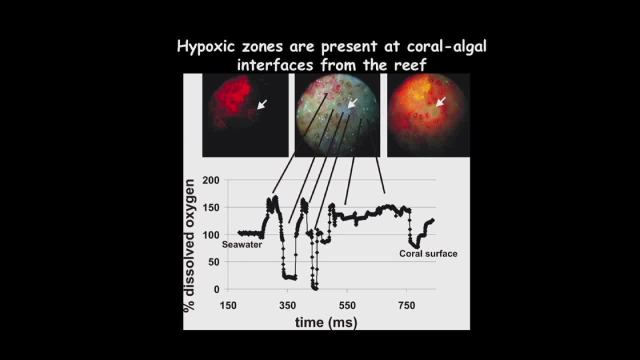 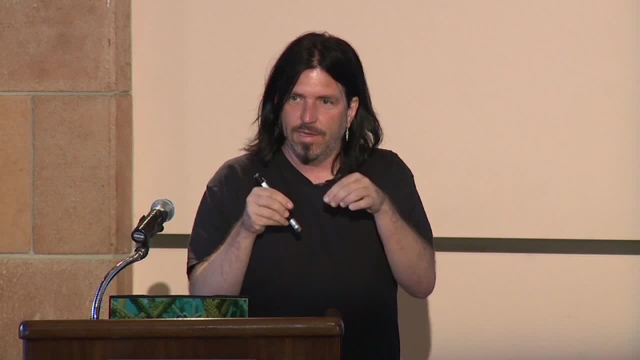 So here's an algae, here's a coral, And if you look where the coral and the algae are next to each other, you actually find these hypoxic zones. So this is where we don't have enough oxygen for the coral And this is how evil the algae is. 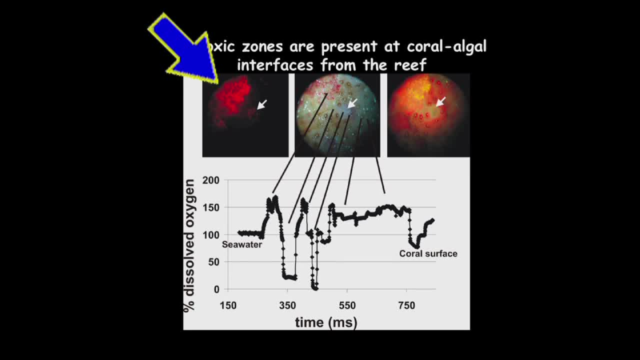 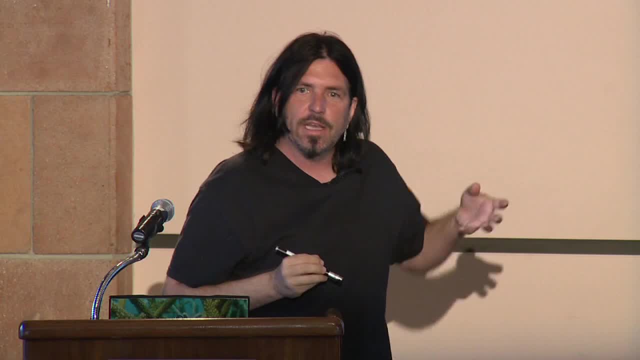 So here's the algae right here. This is a different pigment, Can you see? It's coming in underneath the coral, Okay, And it's forming that little white spot on the coral. So it's coming in from underneath and it's crossing the hypoxic zone. 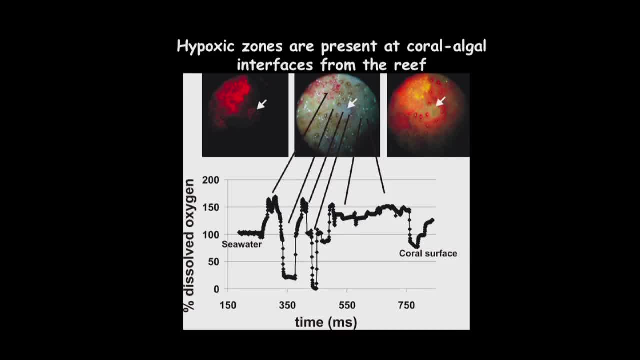 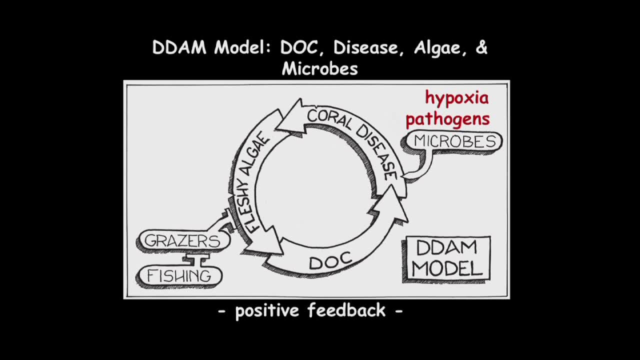 The only time that that happens is when you let the algae grow up so it has more energy to put into those sorts of things, And this is the model. So we call this the DAM model, And the idea is that basically, it's coral diseases that are killing the coral. 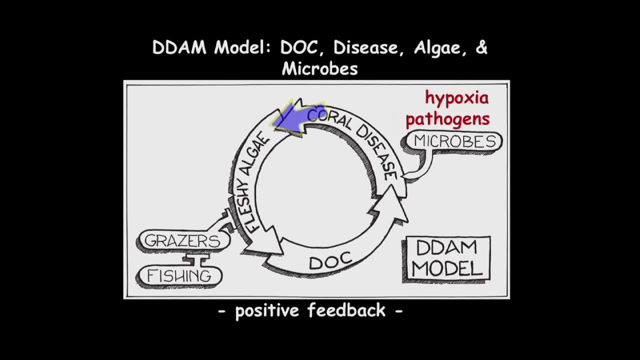 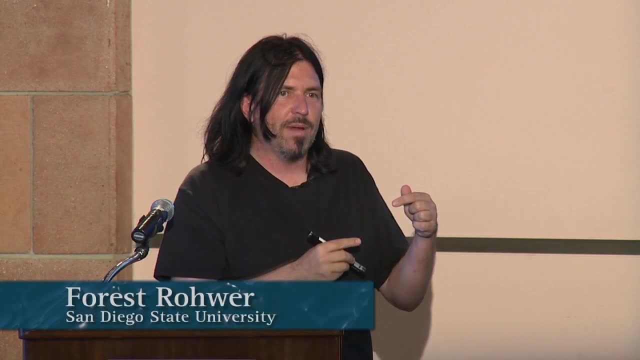 And what they're doing is they're creating more space for algae, And then the algae is producing more of the dissolved organic carbon, which is then feeding the microbes and causing more disease. This ends up causing a positive feedback system, And positive feedbacks are bad because once you get going down them, you can completely 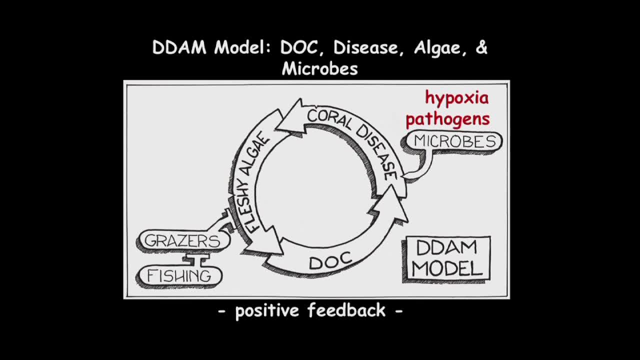 convert one system to another, And what we're doing, of course, is normally we'd have the grazers keeping the algae down, And by fishing we're removing the grazers. The other thing that we can do, which I'll show you in a minute, is we can remove the 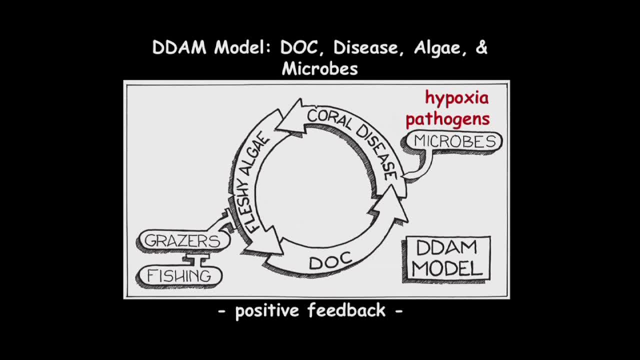 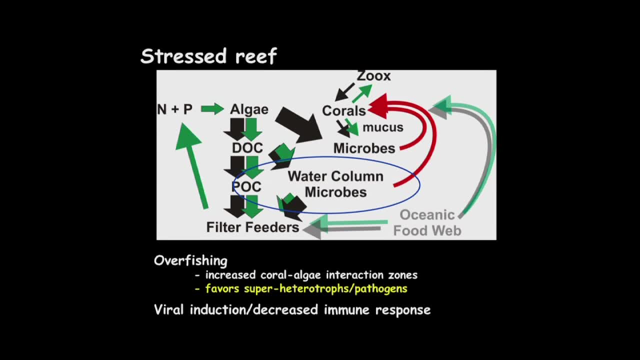 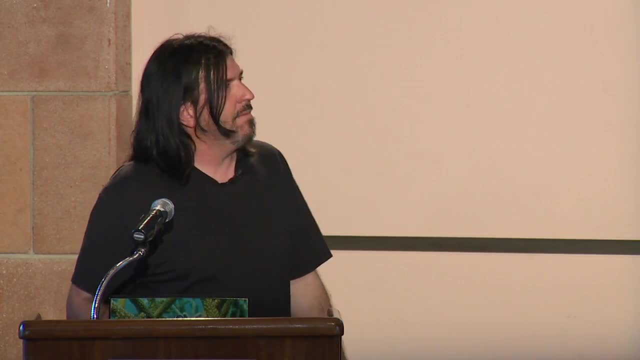 algae. Okay, The other thing that I want to show you in a second is, indirectly, we can feed the algae by adding nutrients to the water. Does this actually happen in big systems, like if we go out and just look in the environment And what we're going to do here is look at the water column, microbes and, in particular, 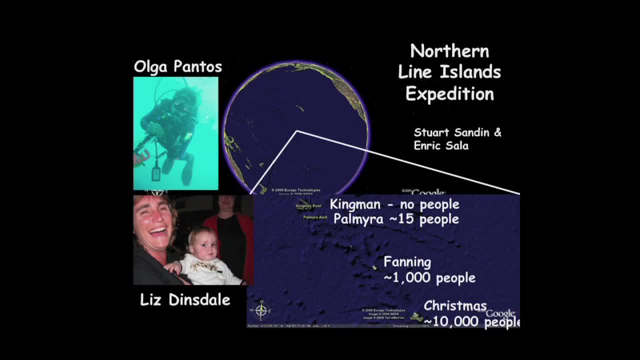 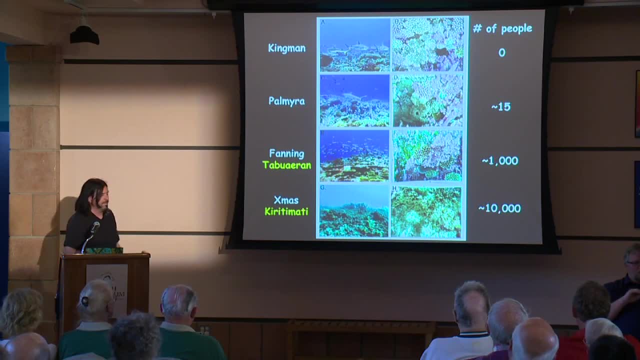 we're going to go to the Northern Line Islands And the four that I'm going to talk about are Kingman, Palmyra, Fanning and Christmas, And they have different concentrations of people on them or different numbers of people on them. 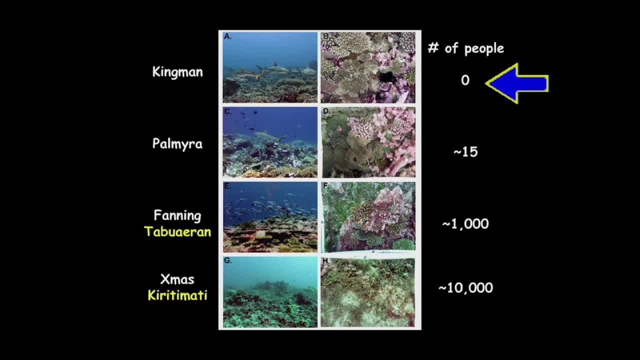 And this is basically what we're doing. This is basically what happens. So here you have no people, you have lots of sharks, you have lots of coral. on the bottom, you have a lot of coral and algae. that's the pink stuff. 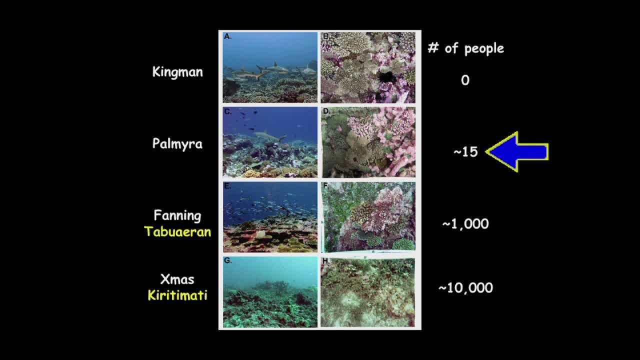 And corals like coral and algae. You have Palmyra, which is a refuge now, but it was fished previously and you're starting to get a little bit more algae in this system. If you go to Fanning or Taberain- it's also called- you can see you've lost all the big 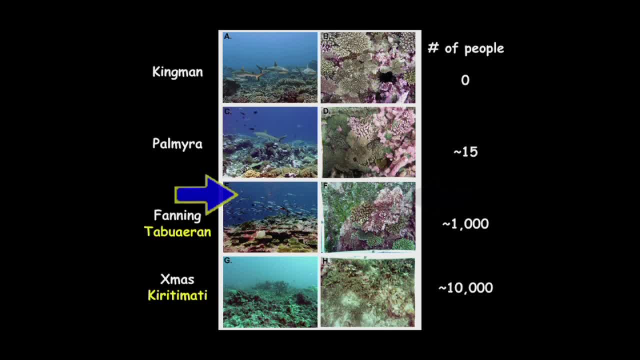 animals right, And all you have are the little fish, And your bottom is starting to shift away from coral to algae. and then you take someplace like Christmas and what's happened is you've gotten rid of essentially all the fish. You just have very small ones. 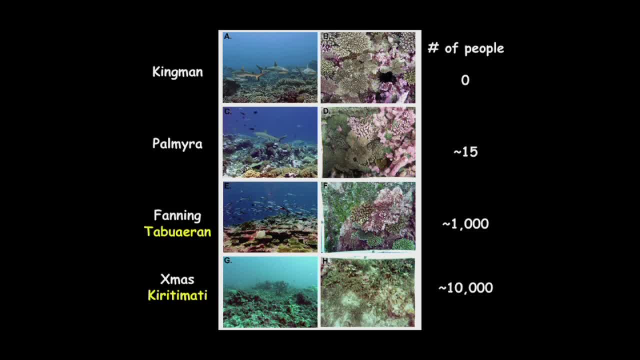 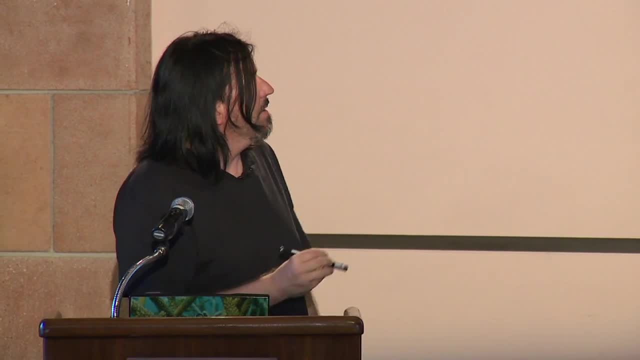 You can see dead coral still standing. so we know that's happened relatively recently. We also did that from other stuff And the bottom has become essentially all algae. This is what happens with the microbes. So the microbes going across. so the Kingman, no people. Christmas with the most people. 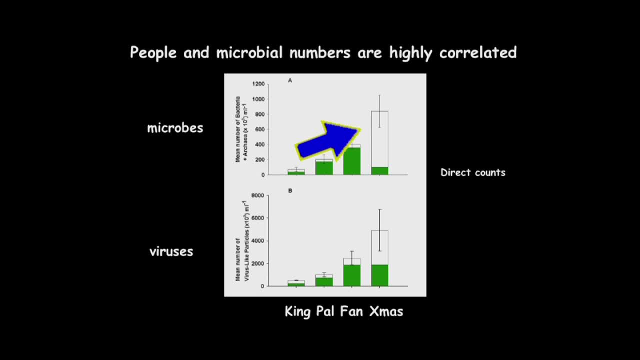 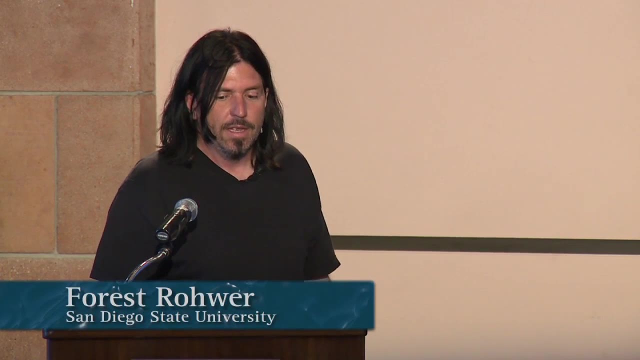 So what you see is the number of microbes here go up by about an order of magnitude, as do the viruses, And most of those viruses are actually the ones that are eating the bacteria. So we see a massive increase in the number of microbes. 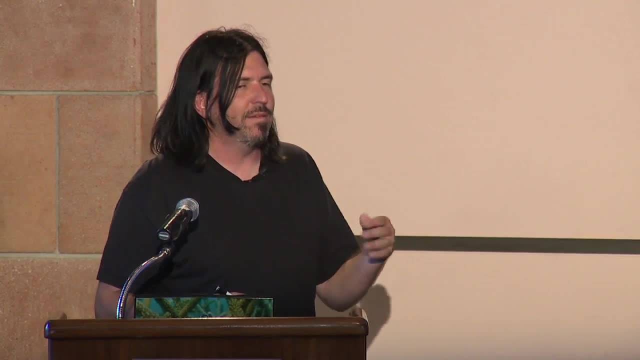 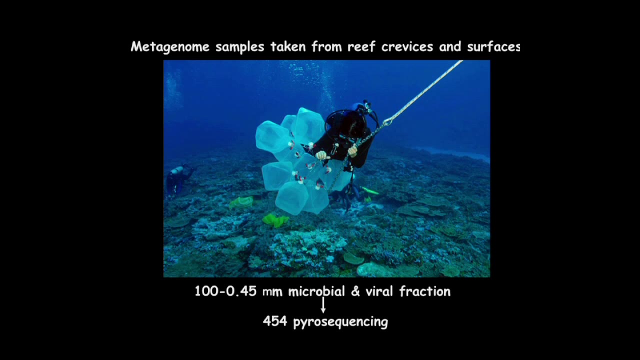 The other thing, though, that we can do, of course, is to figure out what types of microbes they are, using those methods I showed you before. So we're going to go in, collect a whole bunch of water, bring it up and then sequence the 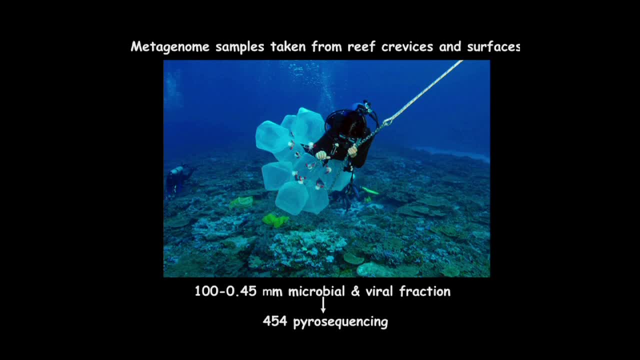 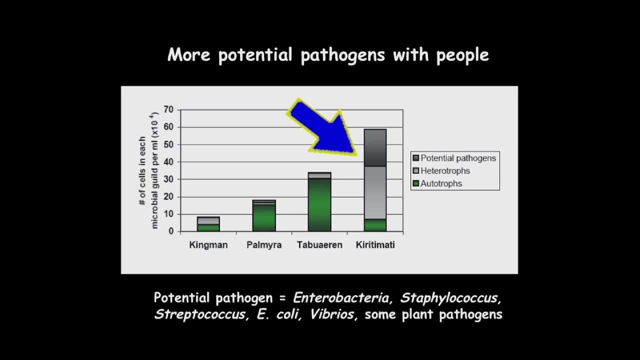 DNA that's associated with them and ask what sorts of microbes we have there. Same thing: here are the four islands. people, no people. You see this increase in the number, but what I really want you to notice is these boxes right here. 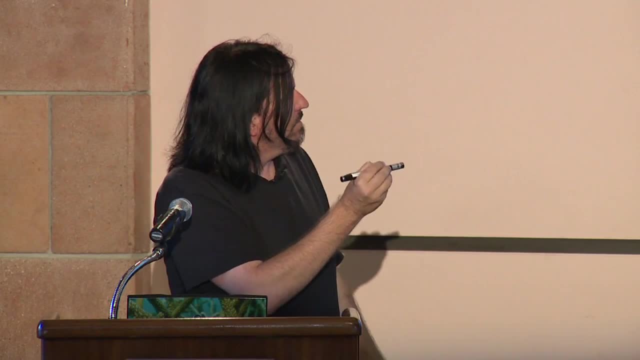 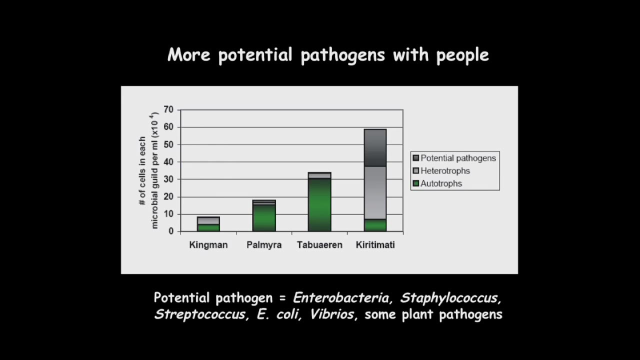 So if you ask, what types of microbes do I have, they've actually switched from. This is what an open ocean community would normally look like, where you have some heterotrophic bacteria. So these are the ones eating the fixed carbon As well as ones that fix carbon. so these are the cyanobacteria to essentially all. 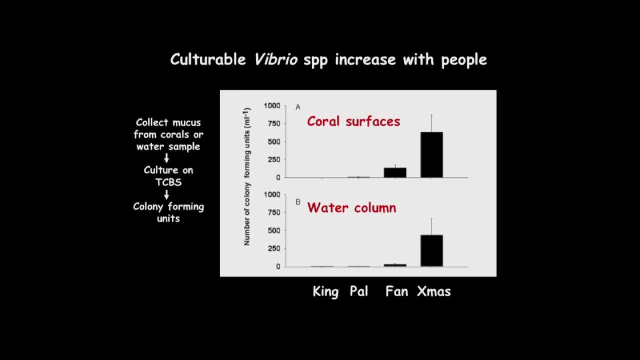 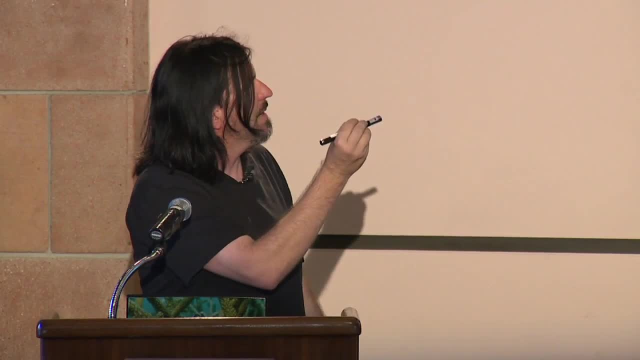 heterotrophic bacteria here. This is another way of looking at it. If you culture, remember, I showed you those microbes that come back and kill the corals. This is a specific group of those microbes And if you look on the coral surfaces you can see without people we essentially cannot. 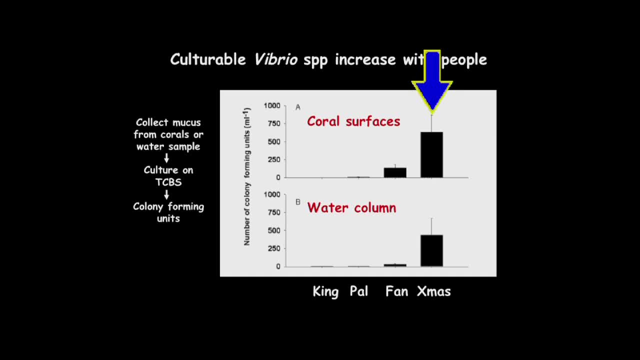 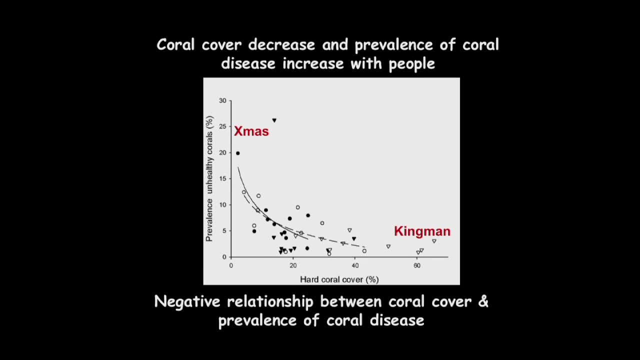 detect any of them, And then, when we get to where we've got the people, you see this increase in the number of them, And then this is probably the final thing that really pulls it all together. What we're looking at here is the amount of coral that we've got on the bottom. 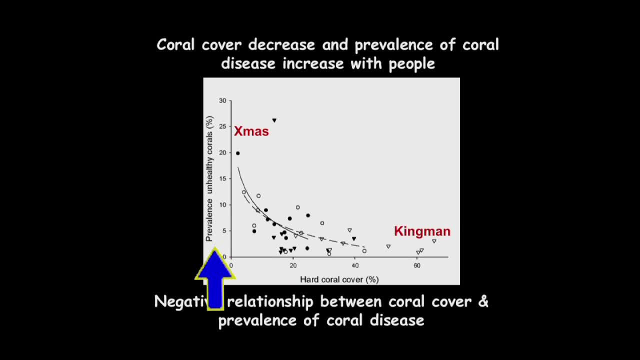 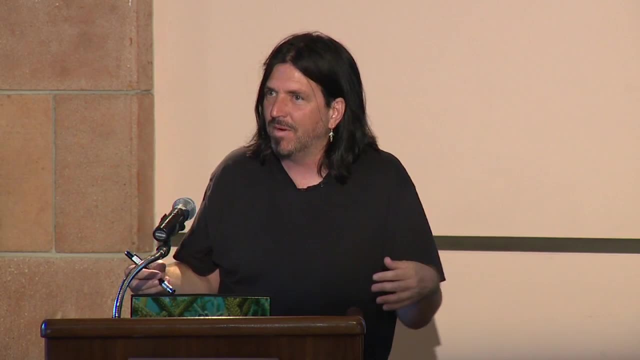 And then this is the disease prevalence going along on this axis, And what I want you to notice is that where we've got more coral, we actually have less disease. Okay, And this looks exactly like what you would expect. Any big population of animals should have a disease incidence of about 5%. 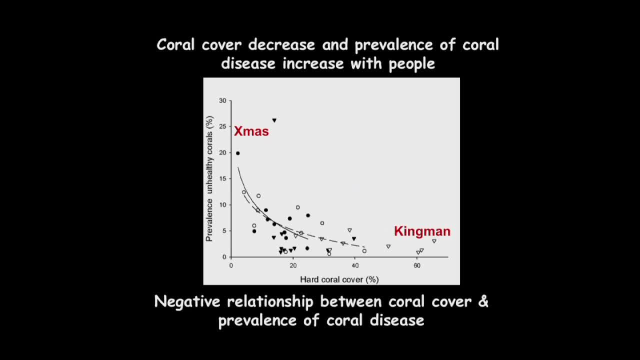 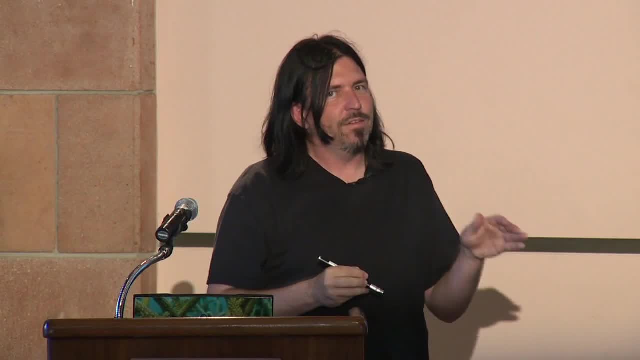 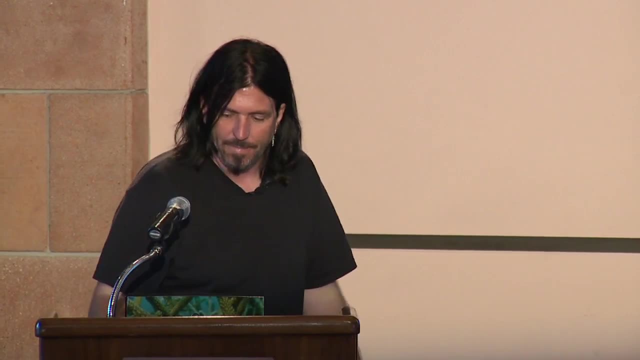 Okay, Which is exactly what we find on Kingman. However, on Christmas, where we have almost no coral left, all of them are sick. That means that you've got something like an opportunistic infection going on, So there's something about that system that's bad for them. 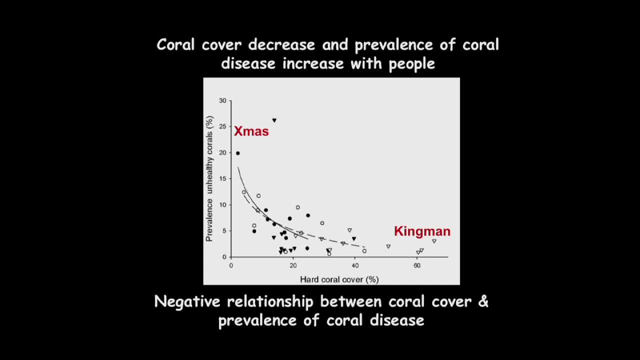 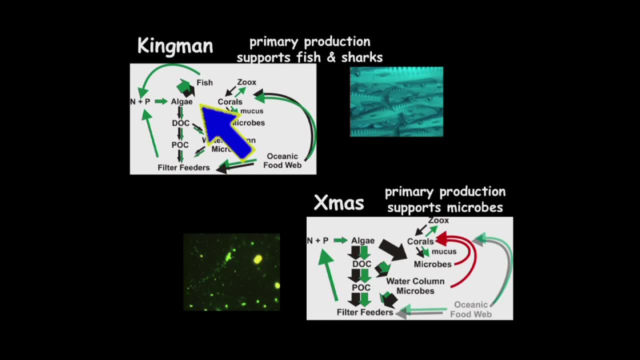 And it's the water quality effectively because of all that extra algae. Taking it all together, what you can say is, someplace like Kingman, most of the primary production, the algae and stuff are feeding the fish And that's why the corals are doing well, because they're able to control the microbes. 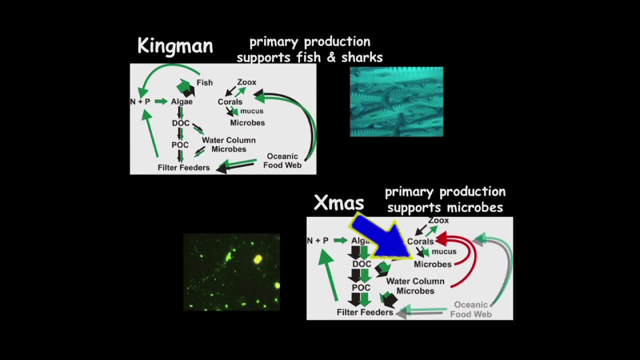 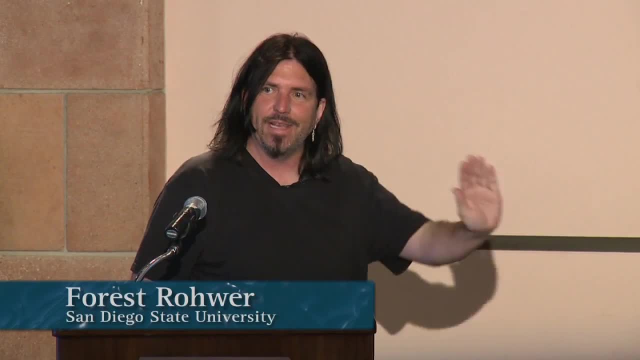 Someplace like Christmas. most of the primary production is actually supporting microbes, And that's what you're seeing there, And what we've found now is that if you look across the whole Pacific Basin, this is happening. It's almost a perfect correlation between people and the number of microbes that we're 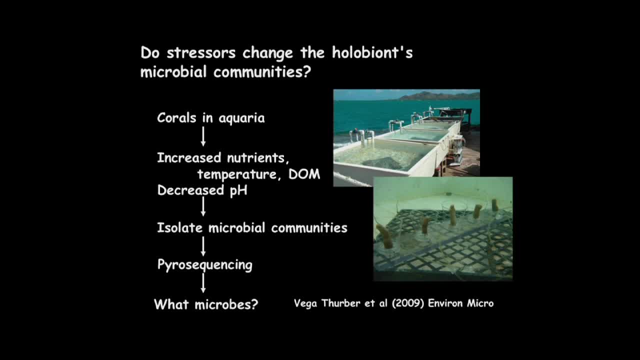 finding in the water. All right, Now let's step back and let's start thinking about the other parts of the holobiont. Okay, So this experiment we've got is corals in an aquarium, And we're going to look at the direct influences of nutrients, temperature and pH on the microbes. 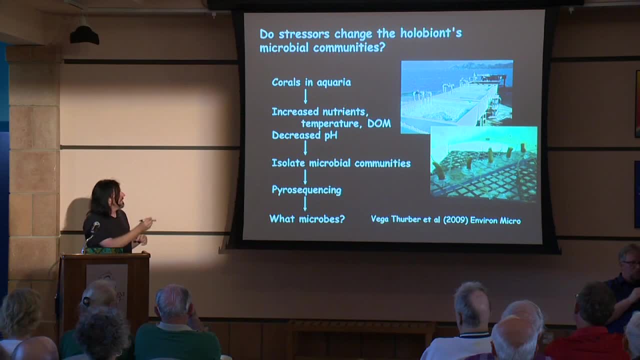 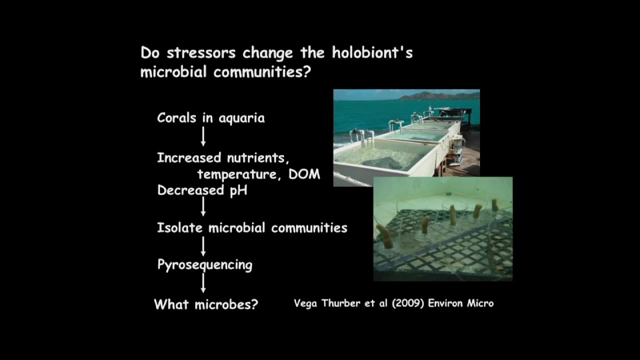 associated with the coral. Remember when we did the culturing before, we didn't actually see that these killed them, But that doesn't mean that they can't be causing problems. We're gonna isolate the microbial communities and then ask: what microbes are there? 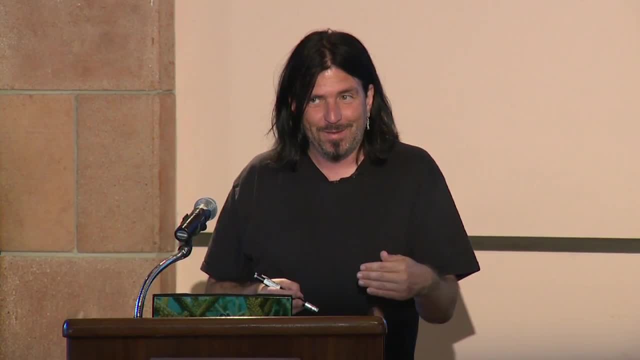 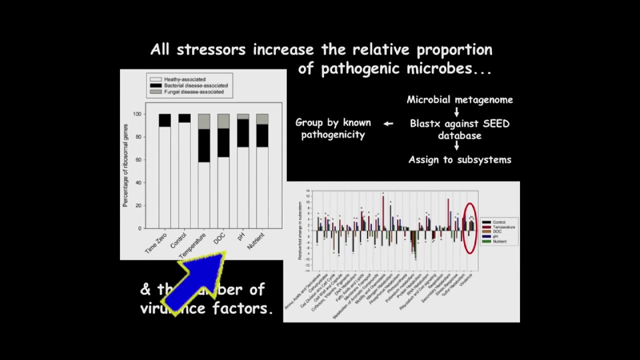 The take home from this is All of the stressors. so anything that we do to a coral in an aquarium like this- So we're gonna do It- doesn't matter whether it's temperature, organic carbon, pH or nutrients- All of them increase the number of pathogens associated with the coral. 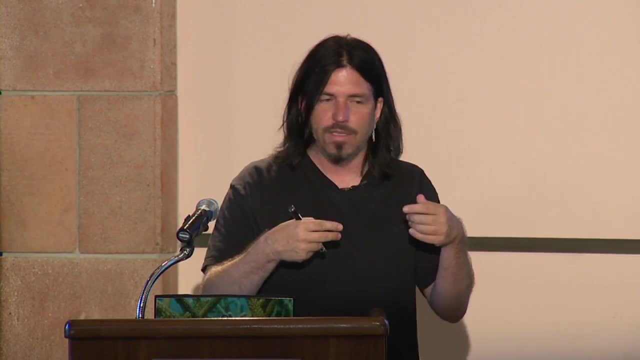 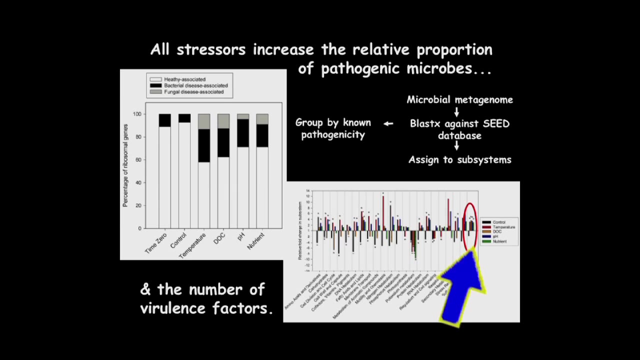 So, even though it's sublethal, we're seeing a change in the associations And you can imagine that over time that actually will lead to coral decline. The more important thing, I think is right here: All of these things actually led to more. 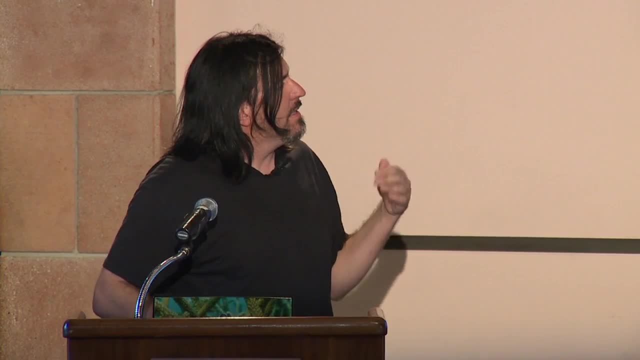 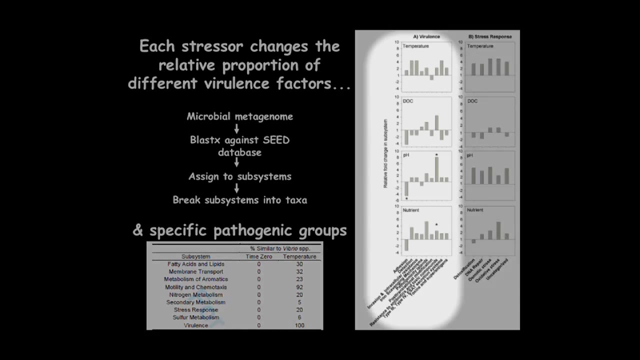 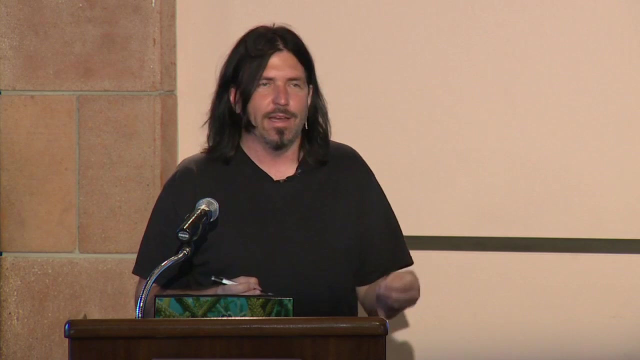 To more virulence factors. Finally, this stuff actually leads to predictive models of what's happening, because you can go in and you can ask of those virulence factors: were they the same across all of the corals and the different stressors, or were they different by stressor? 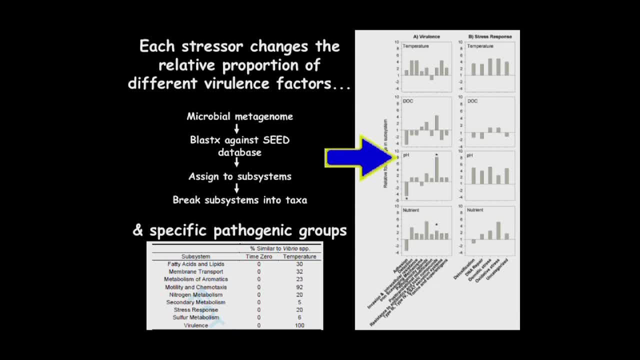 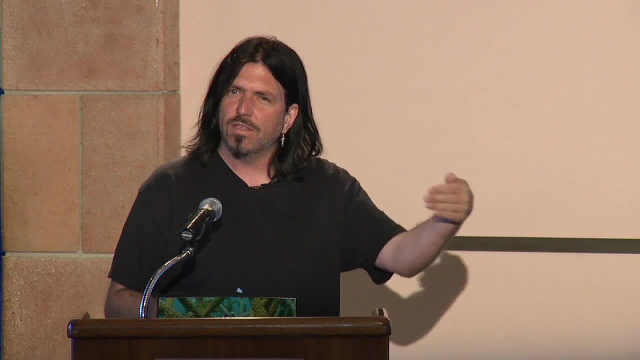 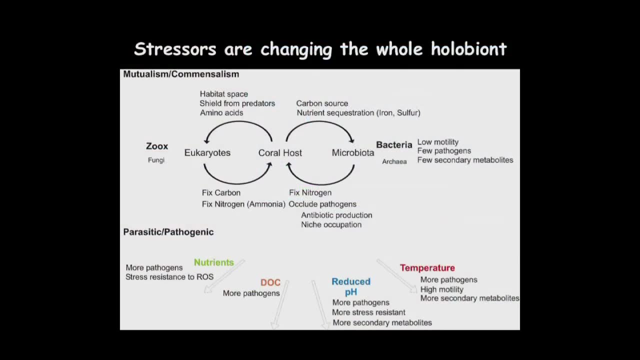 And you can see that temperature has a different pattern than DOC, than pH, than nutrients. So this gives you the ability to go into the system and actually ask What's happening. What stressors are the corals seeing? And taking all of that together, this is just this big model which is horrible to do to. 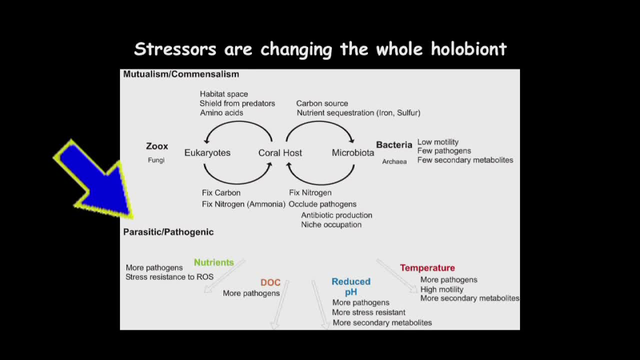 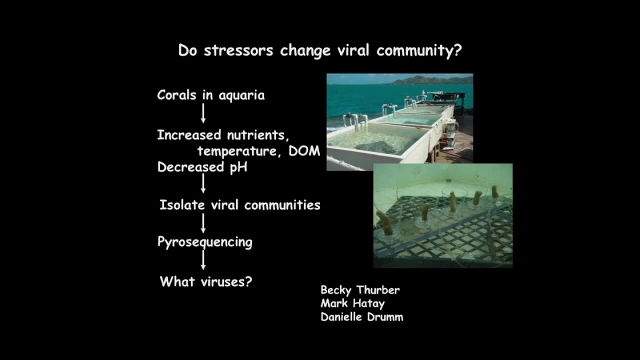 anybody. But this is this idea that any stressor that we add to the coral actually increases more pathogens, and it does it in specific ways that we can predict what's going on. What about the viruses? We're gonna do the same experiment, but in this case we're gonna isolate the viruses. 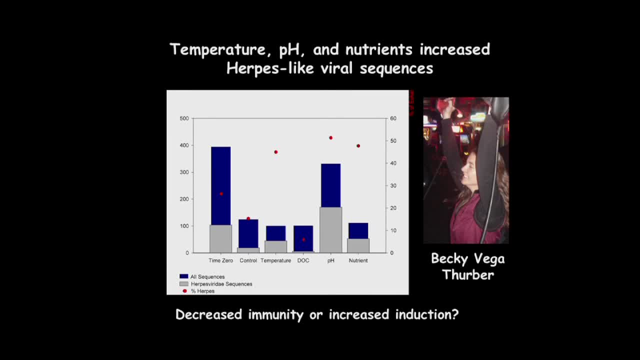 and ask which ones are there? Okay, And the take-home message for this is that three of the stressors- temperature, pH and nutrients- actually induce or cause more herpes viruses to be associated with the coral. What's going on here are these are actually herpes viruses that already are living in? 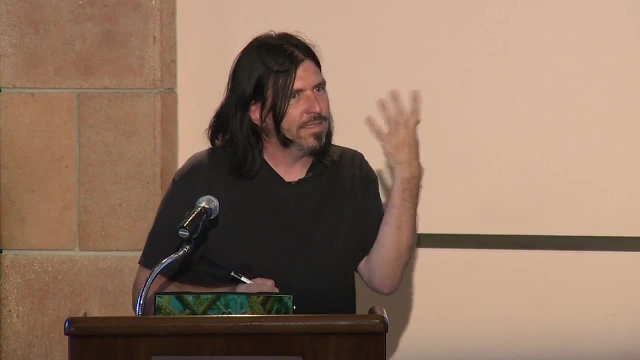 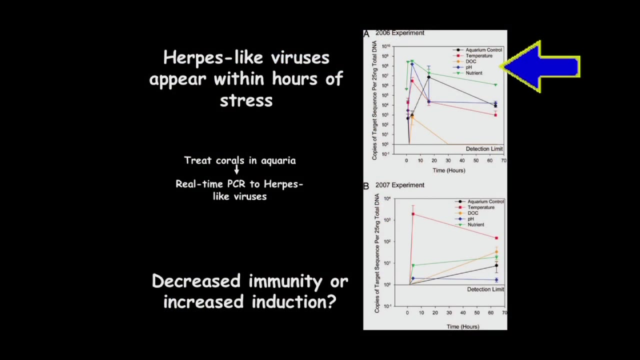 the coral. So, just like you, where you have the herpes viruses that pop out when you're stressed, that's what's going on here And we can actually show that. So if you take the corals and you stress them out with the different stressors, they actually 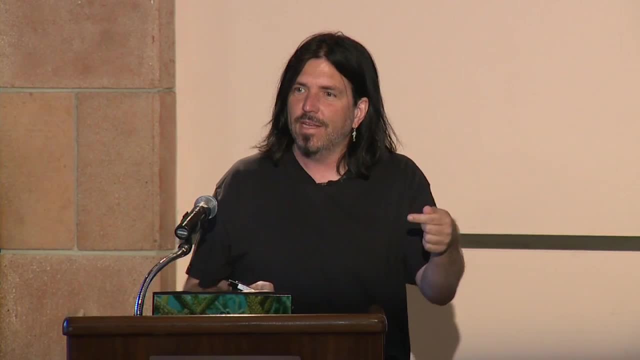 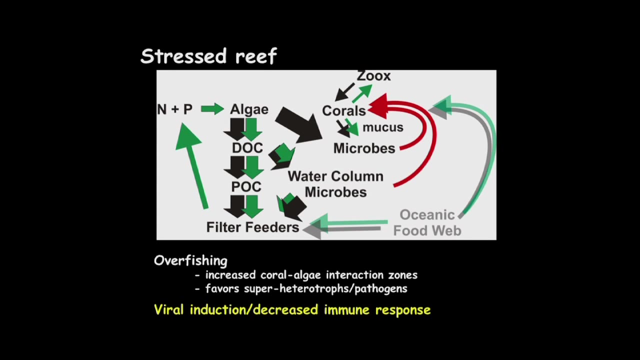 We see more herpes viruses in a matter of hours. So that doesn't mean reinfection, It just means that the ones that are there are already coming out Again. this is one of these other stressors on the system right here, So I didn't want to leave it just totally gloomy. 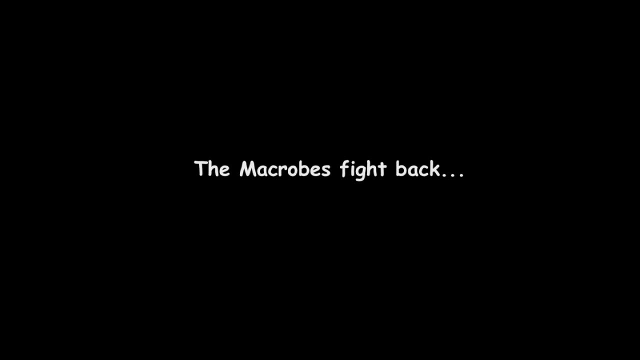 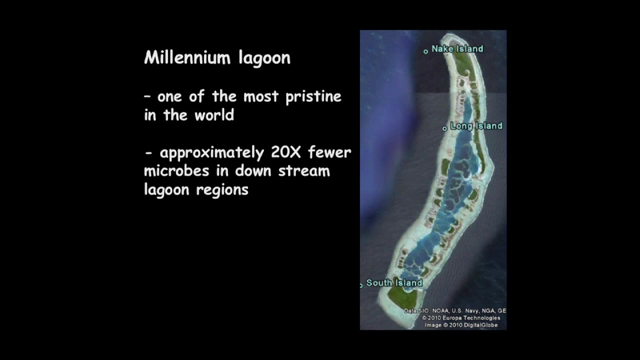 So they get to fight back, And this is one of my favorite places that we go to. It's called Millennium Lagoon. Okay, Millennium is really one of the most pristine systems left on the planet, And what happens in this system is that water gets pushed into the lagoon when the tide 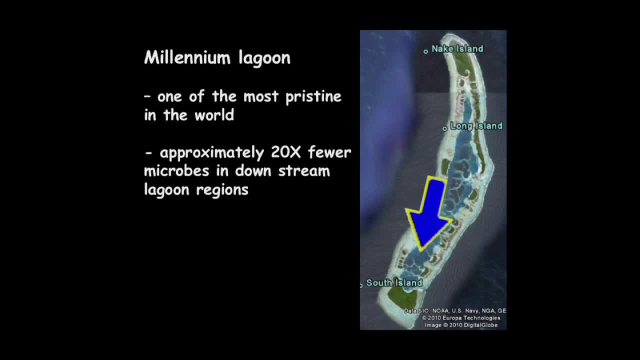 is high and then it rushes out this direction when the tide goes out, and it goes out right here. So the water's moving all the way down this way And you can see that the coral has built these little ribbon reefs across and it's using 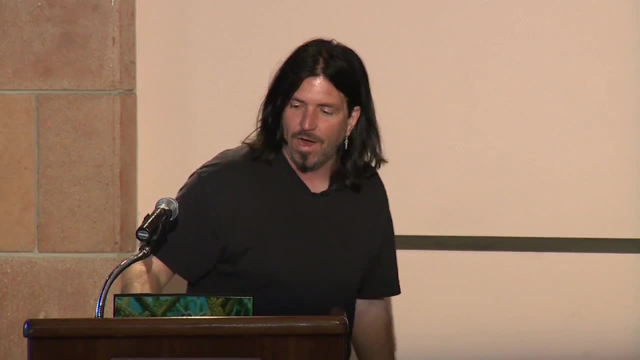 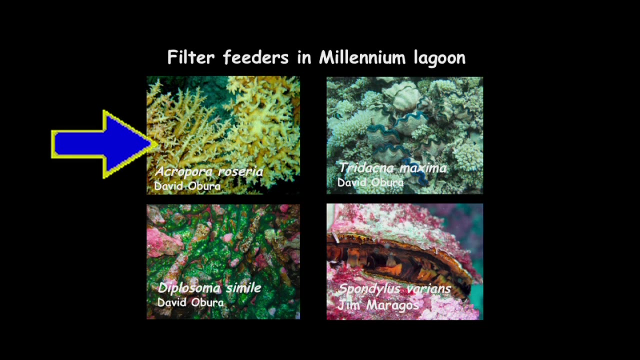 those ribbon reefs to suck out things that are coming down through the water. And these are the ones that are doing it. It's just absolutely beautiful. These are a type of coral. These are the big, the semi-big clams. These are giant scallops. 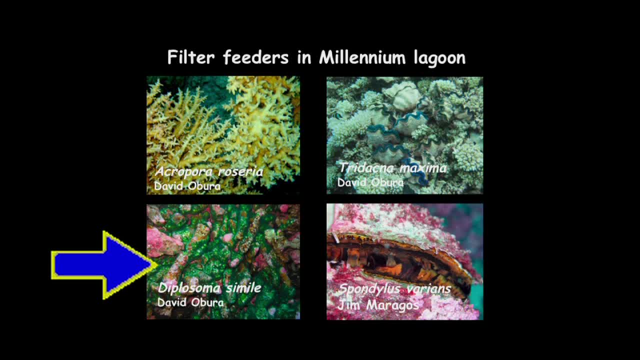 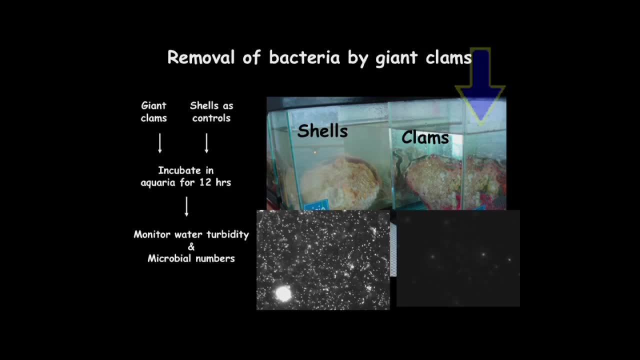 And then these are ascidians, which are a hemichordate, And they're actually sucking all the bacteria out. and this just shows you what happens with giant clams. So if you take a giant clam and you throw it in an aquarium, it eats all the bacteria.